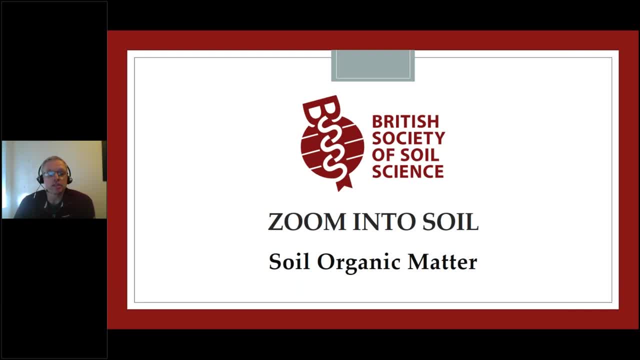 We are an established international membership organization and a charity committed to the study of soil in its widest aspects. We bring together those working within academia and have a growing membership amongst practitioners implementing soil science in industry, as well as those with a keen interest in soils. 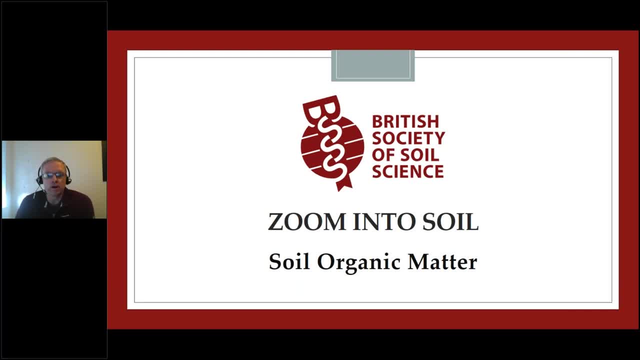 This year we're going to be running 10. Zoom into Soil webinars, and the next one in the series will be hosted by our Northern Soil Network group and that will be on Wednesday, the 3rd of March, on the topic of soil functions, and further information will be distributed after today's event. 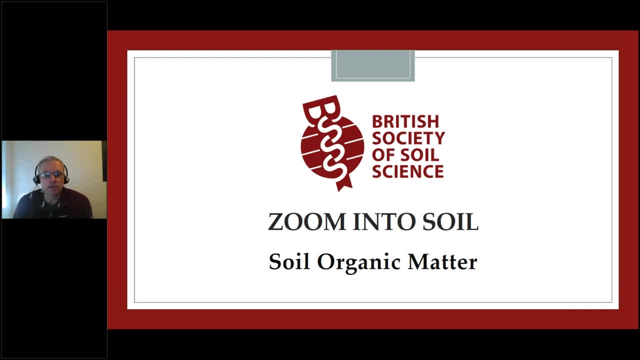 We're also really hopeful that we'll be able to run our two flagship events for 2021 in person later this year. These will be the Early Career Researchers Conference on Monday, the 6th of September, at the Radisson Blue in Glasgow. 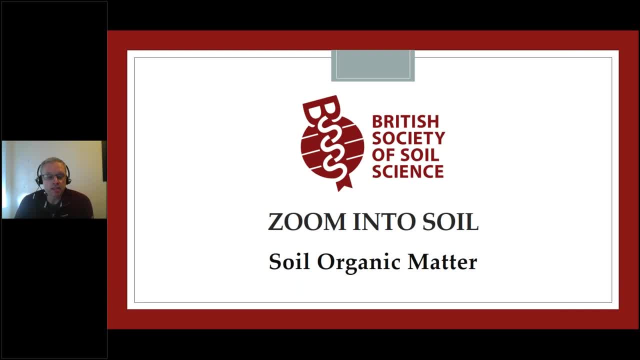 and our annual conference and Gala Dinner, which will be on Tuesday, the 7th and Wednesday, the 8th of September at the Royal College of Physicians in Glasgow. Both of these events will provide an opportunity to hear from invited speakers from diverse soil science specialisms, to see the latest research through oral and poster presentations and also network with colleagues, And again, we're really hopeful that we can do that in person later this year. 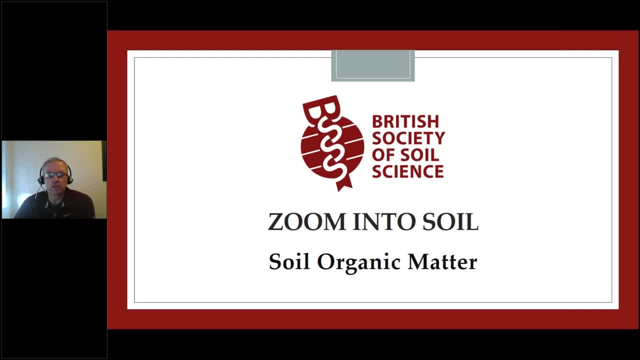 So further information on participating in both events will be available on our website in the coming weeks, And we really do look forward to seeing you there. We look forward to seeing as many of you there as possible and do hope that you'll be able to join us. 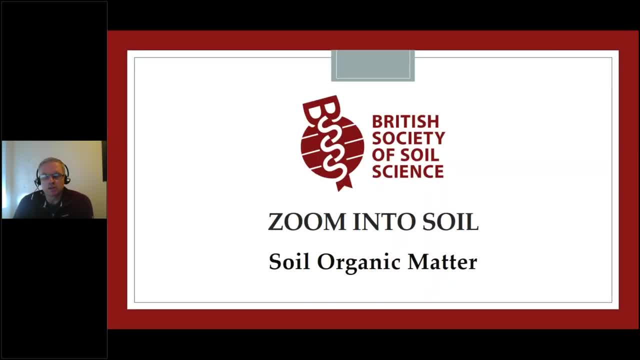 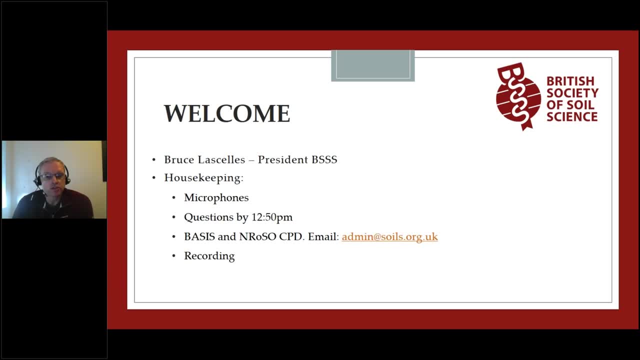 So, just before we start today's presentations, some basic housekeeping. With so many of you here today, all your microphones have been muted. We will be taking questions at the end of both presentations and Tom is going to monitor those for us. 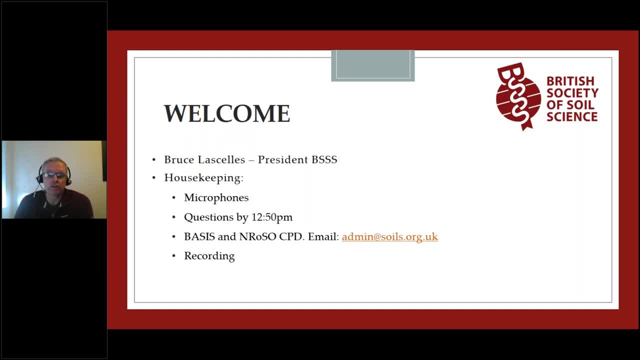 So if you could please submit any questions you've got by 12.50,, that will hopefully allow us to get through as many of those as we can. And whilst on the system there is a raise your hand button, we won't be using this unless the presenter specifically asks for a show of hands. 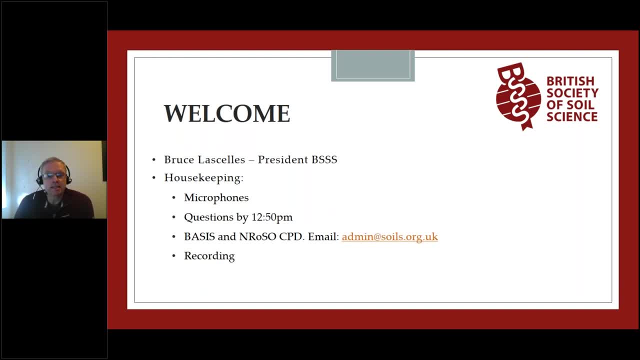 And today's presentations have also been awarded BASIS and NROSO CPD points, So if you're registered with either of those bodies, please contact us directly after the event. And finally, just please be aware that we are recording today's presentation. 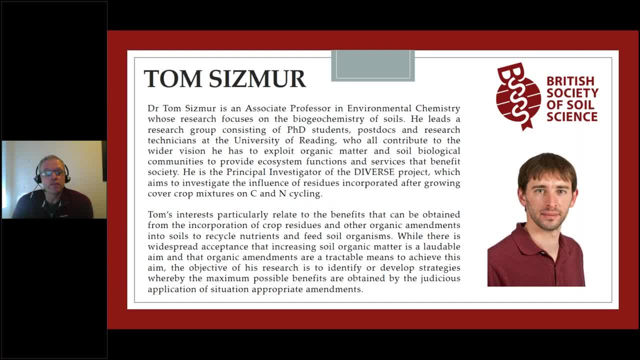 So, moving on to today, I would first like to introduce our first presenter, Dr Tom Zismer. Tom is an associate professor in environmental chemistry whose research focuses on the biogeochemistry of soils. He leads a research group consisting of PhD students, postdocs and research technicians at the University of Reading. 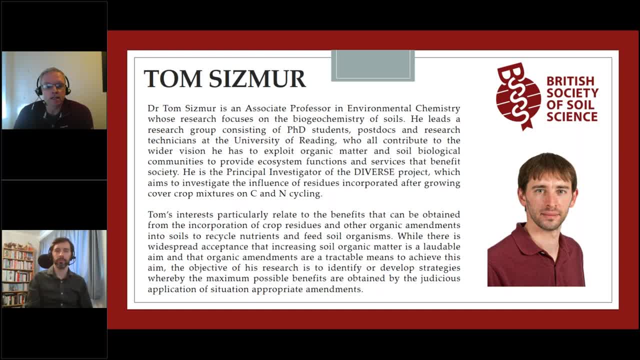 who all contribute to the wider vision he has to exploit organic matter and soil biological communities to provide ecosystem functions and services that benefit society. He is the principal investigator of the DIVERSE project which aims to investigate the influence of residues incorporated after growing cover crop mixtures on carbon and nitrogen cycling. 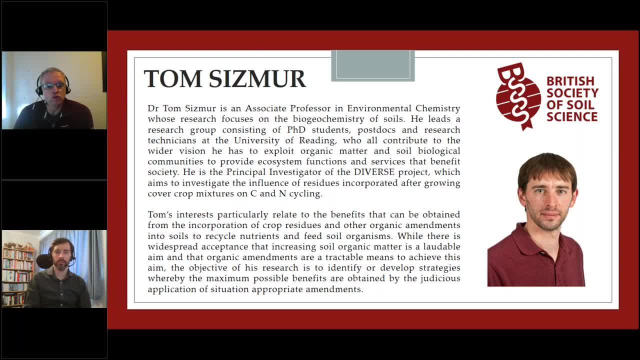 Tom's interests particularly relate to the benefit that can be obtained from the incorporation of crop residues and other organic amendments into soils to recycle nutrients and feed soil organisms. Whilst there's widespread acceptance that increasing soil organic matter is a laudable aim and that organic amendments are an attractable means to achieve this goal, whilst there's widespread acceptance that increasing soil organic matter is a laudable aim and that organic amendments are an attractable means to achieve this goal. whilst there's widespread acceptance that increasing soil organic matter is a laudable aim and that organic amendments are an attractable means to achieve this goal, 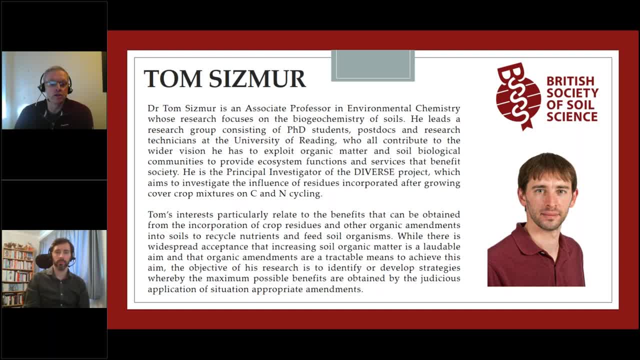 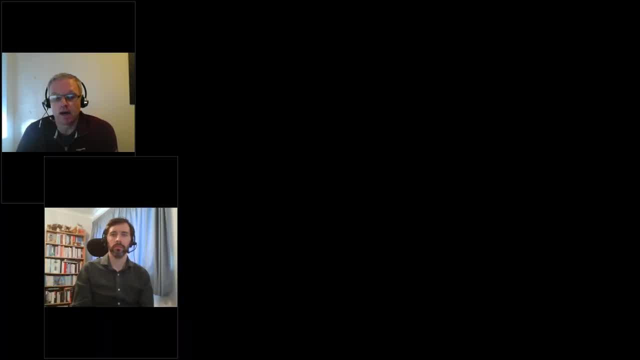 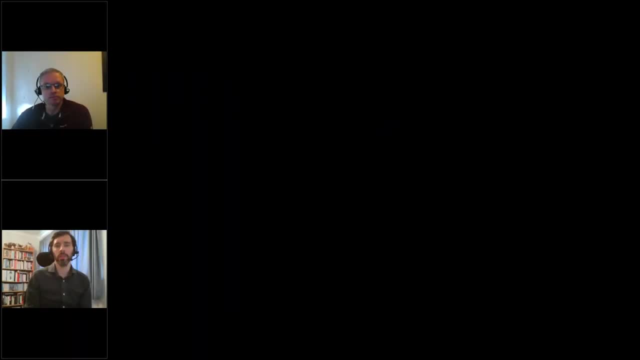 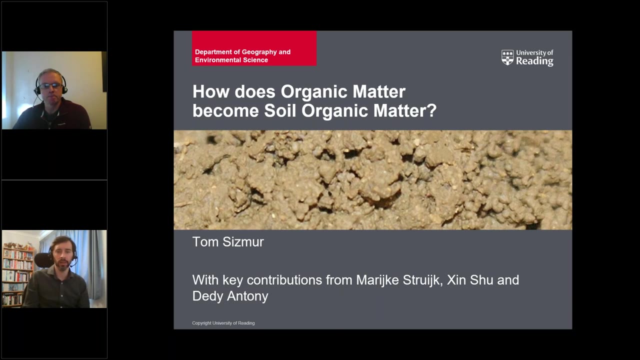 the objective of his research is to identify or develop strategies whereby the maximum possible benefits are obtained by the judicious application of situation, appropriate amendments, And so, with nothing, formerly over to you, Tom. Thank you very much, Bruce, So I'll just share my screen now and hopefully you can see it and continue with my presentation. 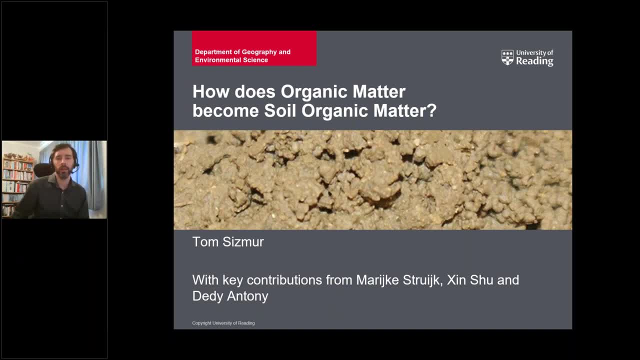 So I'm Tom Zismer. Thank you very much for the introduction and good afternoon And to everyone. I'm just experiencing a few issues. I think I've got my presentation shared now, So do come back on, Bruce, if it's not, if it's not showing. 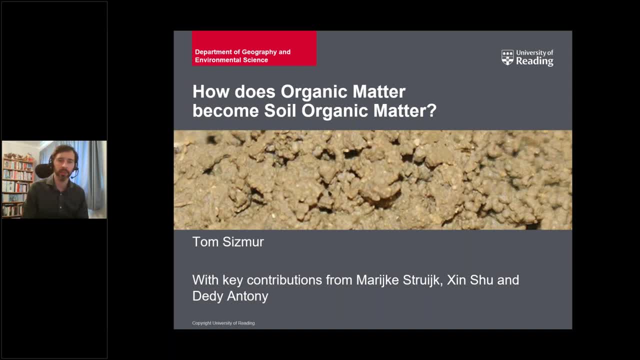 So I'd just like to say that today's presentation is a collaborative effort. So it's not just me but also sort of several members of my research group that have contributed to the stuff I'm going to share here, In particular Marika Strauch and Shinshu and Deddy Anthony who've kind of contributed sort of slides or data that I'm going to be sharing with you today. 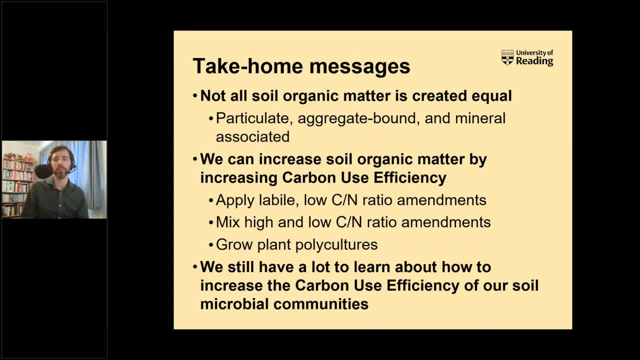 I just wanted to start here with my take home messages for today's presentation, And so, first of all, I'd just like to say that not all soil organic matter is the same. It's not all created equal, And I'll introduce you to three different key groups of organic matter within soils. 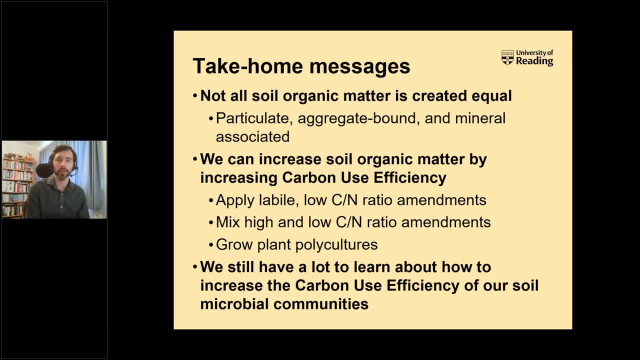 So part one: soil organic matter, particulate organic matter, aggregate bound organic matter and mineral associated organic matter. And then I want to introduce you to the concept of carbon use efficiency of the microbial communities in soils and how this can be manipulated in order to increase the 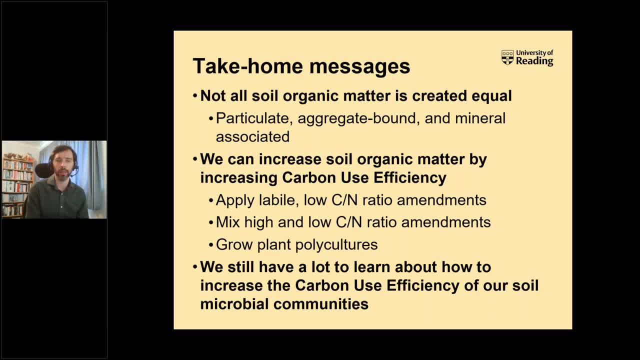 amount of organic matter that becomes stabilised in soil and a few strategies that we might want to employ in order to increase that stable organic matter in soil. So applying labile low carbon to nitrogen ratio amendments, perhaps mixing high and low carbon to nitrogen ratio amendments, and growing plants in polyculture. So we've got diverse amendments going to the 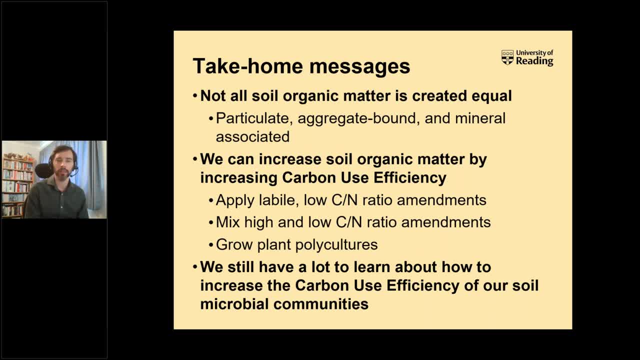 soil, And then at the end, I also kind of want to highlight that this is a bit of a journey that we're on and that we've still got quite a lot to learn. So I kind of want to share with you some of the sort of things that I'm thinking about at the moment as to 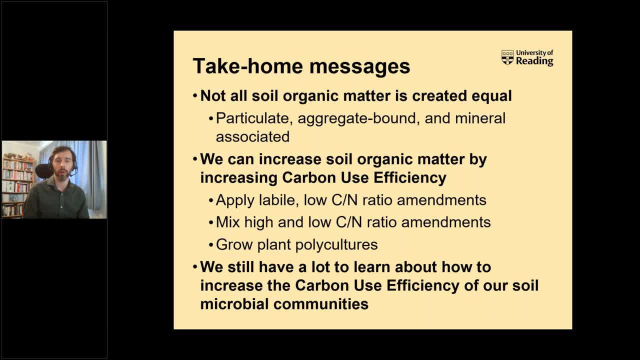 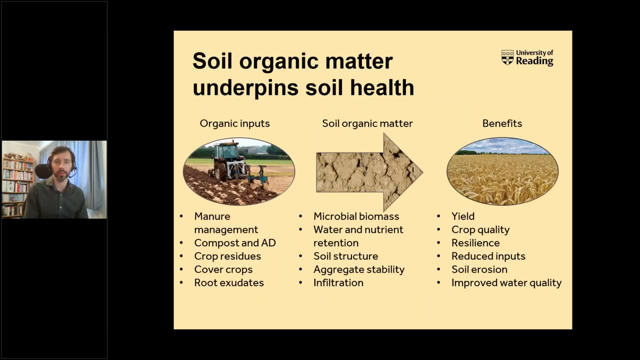 how we can then advance our knowledge Of how we might be able to exploit microbial carbon use efficiency of our soil microbial communities to help build soil organic matter. But first of all, just a bit of an introduction to soil organic matter, So what it does for us and what benefits we can obtain from it. 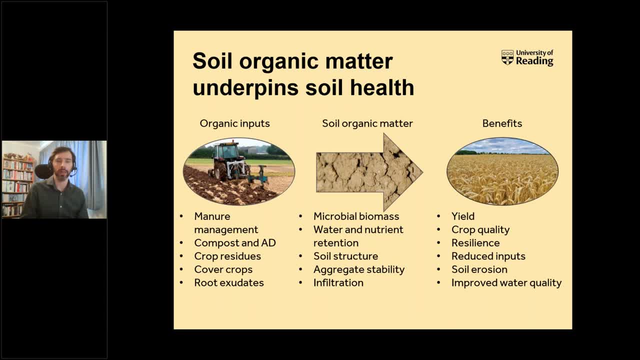 And there's a number of different ways in which we can build soil organic matter in soils by adding organic inputs, So we can add manures, for example. We can add other soil amendments, like composts or anaerobic digestates. We can return the residues of crops into soils. We can grow cover crops in between cash crops. 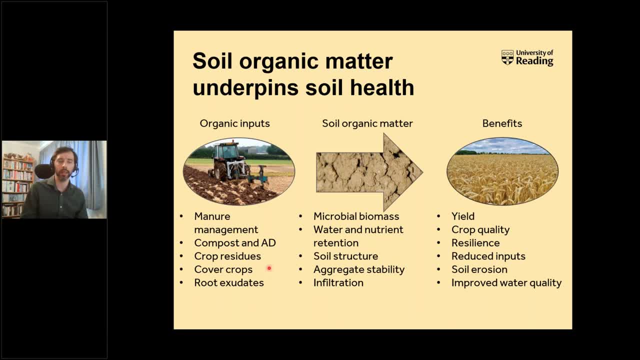 as a way of growing, having more plant material that we can add into the soil, And also all of these crops and plants that we grow in our soils will be releasing root exudates, That's carbon that's being pumped down into the soil from the plant. 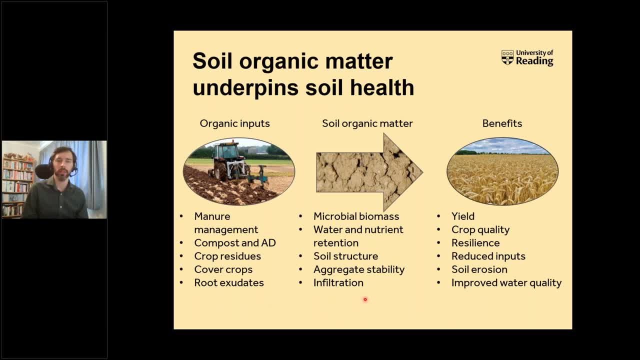 And so what sort of functions does this organic matter then provide? Well, it's, very importantly, a food for not just the microbial biomass but for the entire soil food web, which themselves provide a lot of functions and services. So our soil organic matter helps our soils to retain. 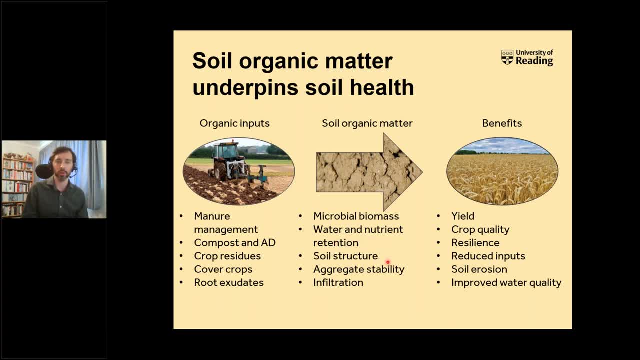 water and nutrients. It helps benefit our soil structure And ultimately, this crummy sort of soil structure that you get through these stable aggregates that are stabilized by the presence of the carbon, helps our soils infiltrate water and helps to store water. Ultimately, the benefits. 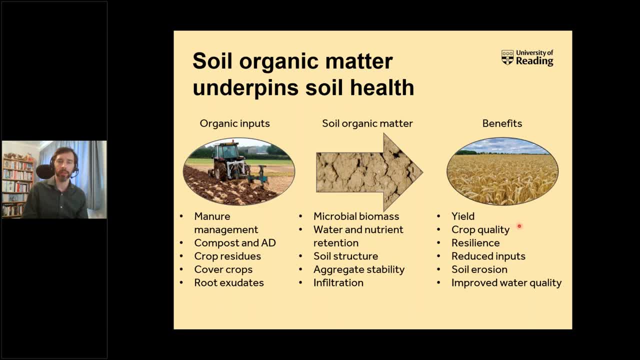 to land managers are that we get improved crop yield and quality, We create soils that are potentially more resilient to extreme weather events, And we also are able to grow more crops with reduced inputs. So we're able to increase the efficiency of our crops. So we're able to increase the efficiency of our crops. 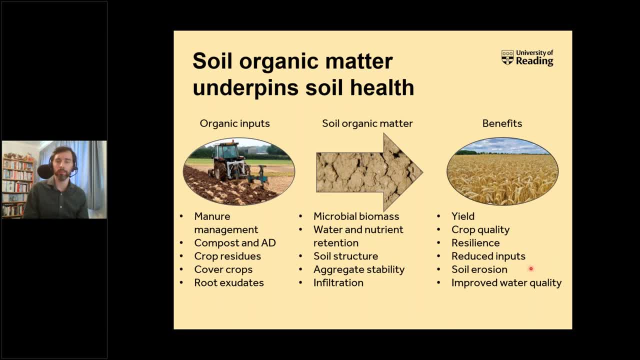 And, ultimately, that soil. organic matter helps to bind the soil together, preventing erosion and ultimately improving the quality of our water, both because there's less nutrients leaching through the profile and also less soil running off of our fields into rivers. But the thing that I want to focus mostly on today is how does organic matter so the organic? 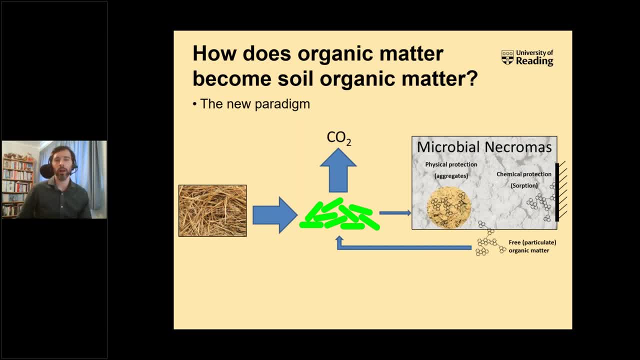 matter that we apply to soils or that enters soils. how does that become soil organic matter? How does that become soil organic matter? And until about sort of 10 years ago or so, the sort of the prevailing belief was that soil organic matter was essentially. 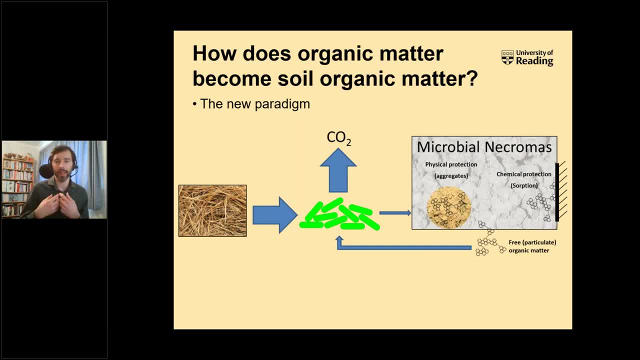 undecomposed plant material, So plant material that had been entered into the soils, which then plays a little bit of a game of luck whereby some of that is decomposed and some of it isn't, and perhaps some of the more recalcitrant compounds were believed to be those things. 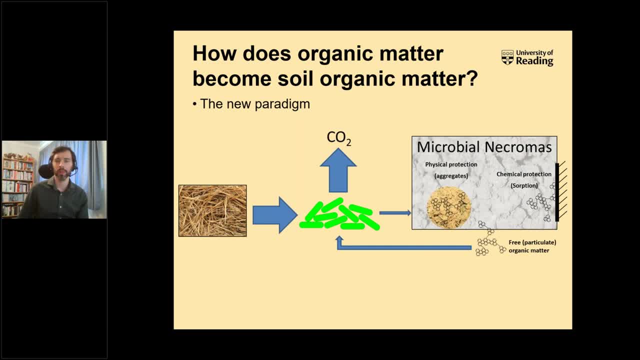 that remain stable in soil for a long period of time Now, over the last sort of approximately 10 years, that our paradigm has shifted. So our understanding of how soil, organic matter is created in soils has changed a little bit, And I'll sort of briefly describe the sort of the 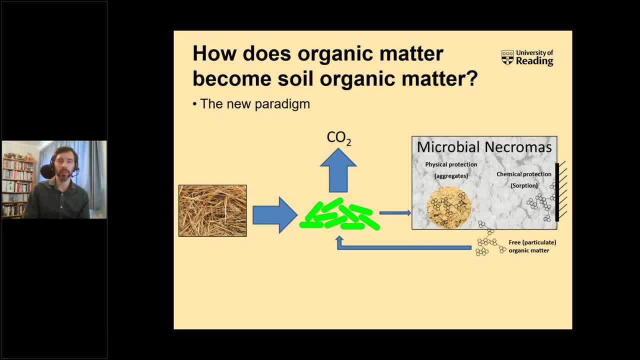 major processes using this diagram here. So I appreciate that this is limited very much to the extent of my artwork capabilities. But this over here, this picture of this straw, represents kind of all plant litter that might then enter into soils, And what we now know to be true is that 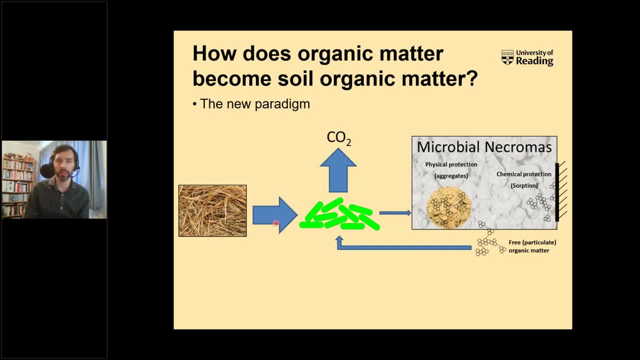 the majority, the vast majority of that plant litter is decomposed, I should say goes into the microbial community, is decomposed by the microbial community and in fact the entire soil food web in a relatively short period of time. And then again the majority of that carbon. 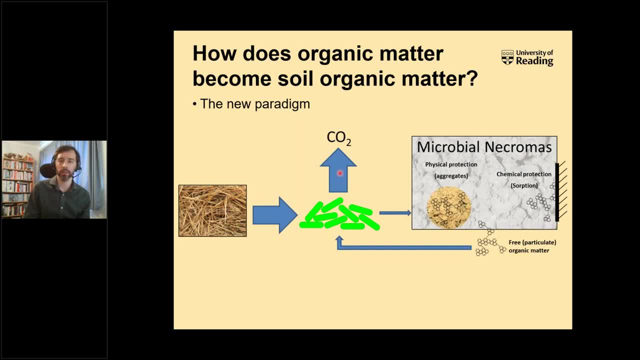 that comes in then leaves the system as carbon dioxide, And occasionally it's methane, for example. But then a small amount of that carbon is then stored as biomass in that microbial community And eventually that microbial community will die. So microbes will die. 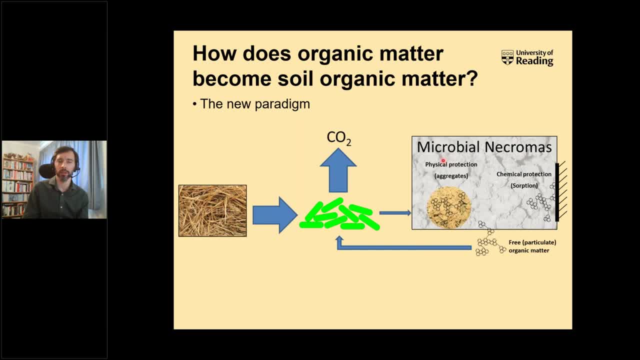 And those microbes will then become the microbial necromass, so the dead microbial community, And there that's the stuff that typically gets stored for a long period of time in soils And there's two primary mechanisms that it gets So it can become physically protected within aggregates. So there's an aggregate that 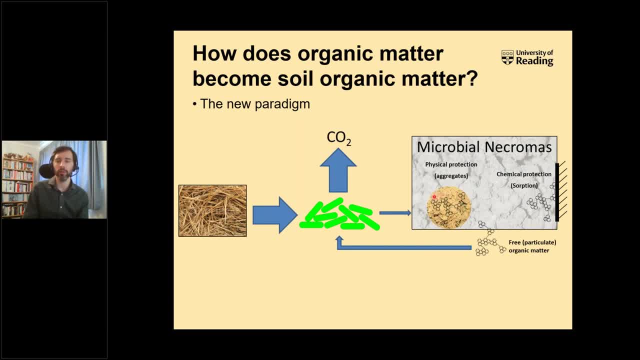 physically separates that dead organic matter from the live organic matter that might gobble it up and eat it. Also, it can become chemically protected as well. So it can basically become stuck to a surface of a soil through sorption processes And because it's stuck to that surface, it's 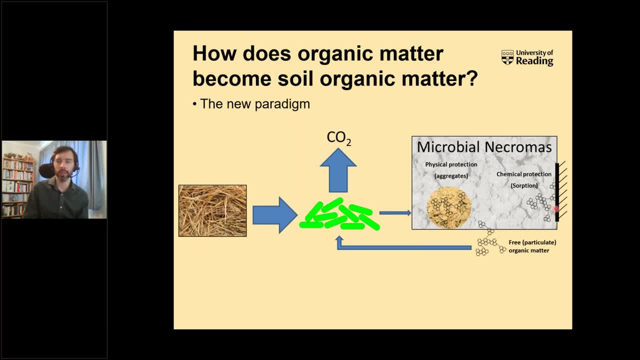 not able to then dissolve into the soil solution and become again ingested by a soil microbe. But over time we do get some desorption and we do get these aggregates breaking up, And so some of that organic carbon will then become what we call that free particulate. 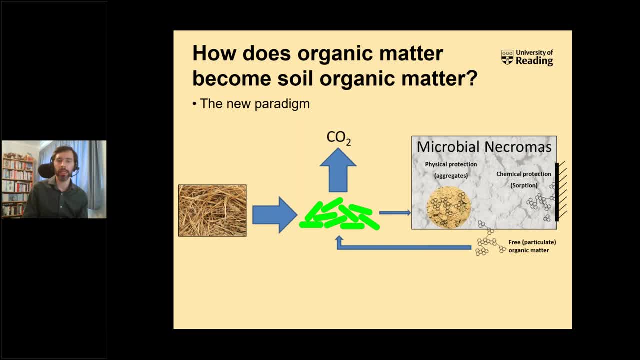 organic matter. And so these three kind of key pools- the physically protected organic matter, the chemically protected organic matter and that free particulate organic matter- form the three kind of primary pools of organic matter in the soil environment, And then the system basically keeps cycling around so that 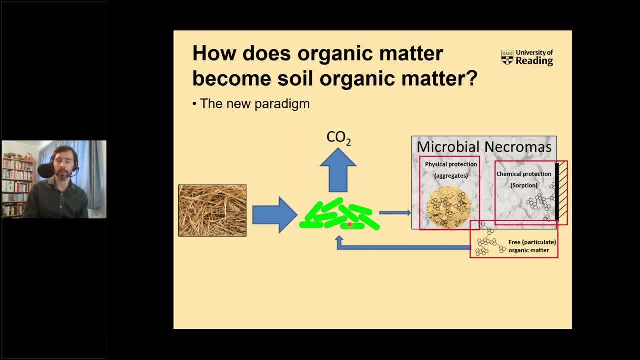 organic matter that can become free again comes back to the soil biological community, And again we can play that game again. where some of it will be retained in the biomass, Much of it will be released as carbon dioxide. But of the bit that is retained in the biomass, 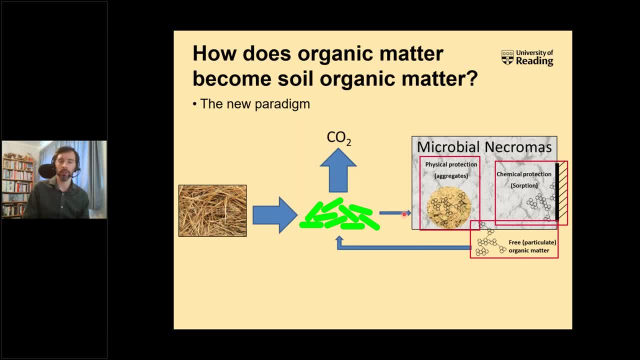 that can then become necromass and dead microbial matter, which then can become stabilized in the soil Again, and so the stuff that is really old, the organic matter that's been in the soil for a very long period of time, may have gone round this cycle on multiple occasions, And so it's pretty. 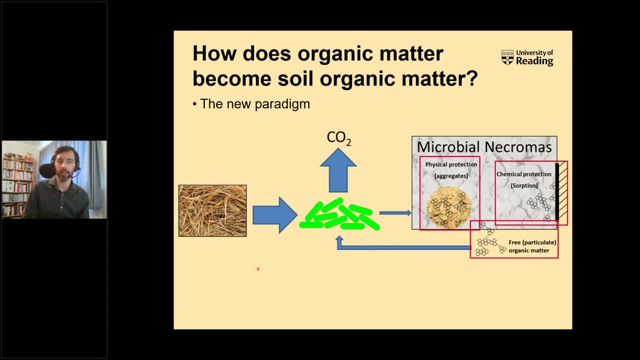 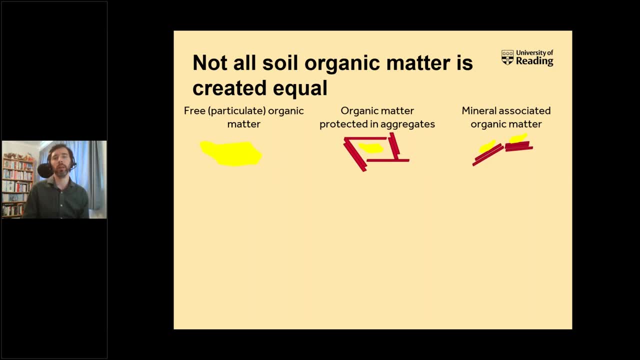 unrecognizable from the stuff that originally entered into the soil. Now I'm going to focus a little bit more on these three major groups or major classifications of soil organic matter in the soil- And we've got that free particulate organic matter, the organic matter that's protected aggregates and the organic matter that's associated. 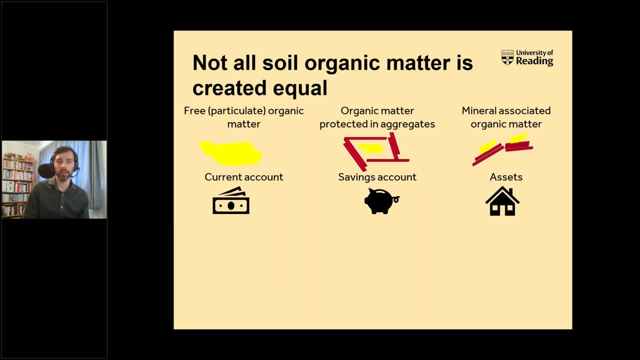 with minerals And just by way of analogy, I would use the analogy of kind of money or finance to classify these things. So your free particulate organic matter is a little bit like your current account or the money that you might have in your wallet at any given time. 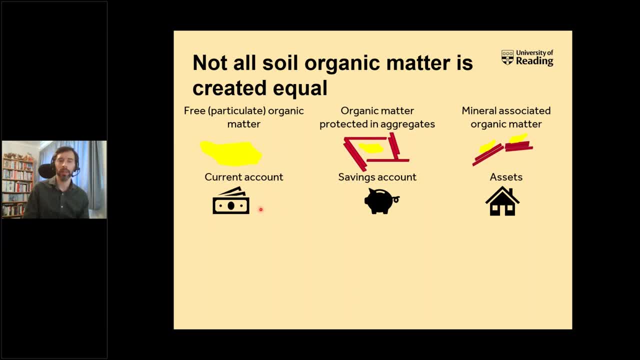 So the turnover of this free particulate organic matter is pretty rapid, So it doesn't last very long in the soil. It gets gobbled up by microorganisms and other members of the soil food web And, as a result, we need to keep replenishing this pool of organic matter. 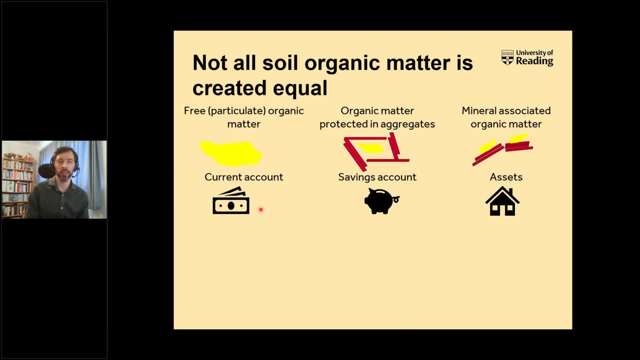 if we want to build up a store of it in order to perform some of the functions that we want our soils to perform: The organic matter that's protected aggregates- I would maybe use this as a bit of an analogy- of your savings account. So this is your. 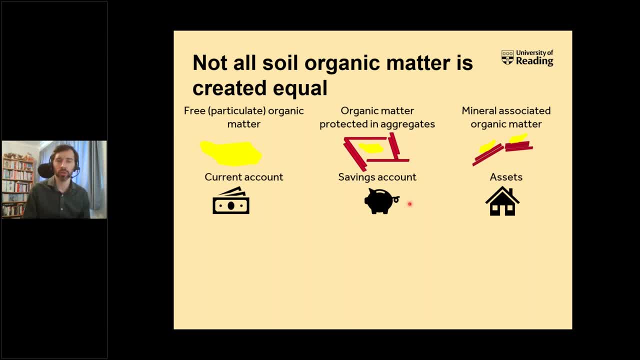 relatively long term store of carbon in the soil, But it's also quite easy to blow your savings account. So if you have a bit of an issue and you need to spend a bit of money quickly, then it's quite easy to lose all of that carbon. Mineral associated carbon. 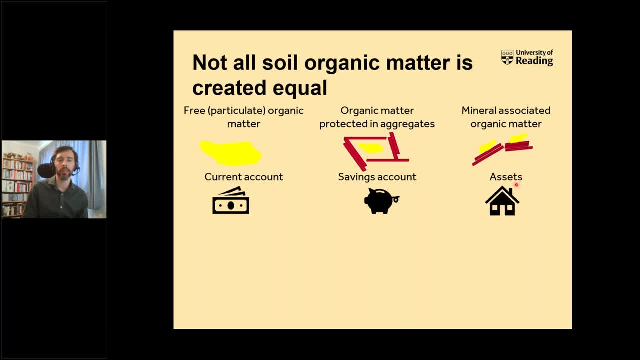 I would use as an analogy of: like your assets, So this is your long term store of finance. It's actually a lot harder to get rid of this store of carbon in the soil than it is the other two versions, But equally it takes a very long time to build up those assets as well, So it takes a. 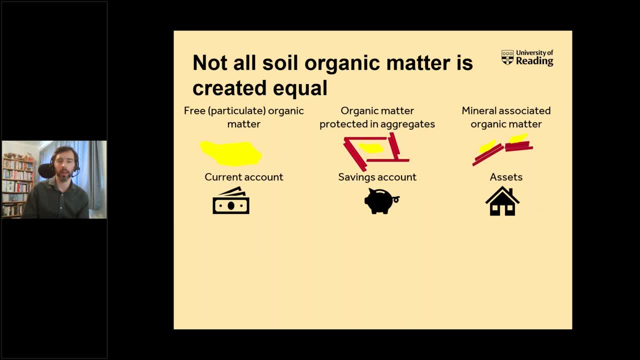 very long time to build up that mineral associated organic matter in the soil. So what functions do these different pools deliver? So the free particulate organic matter. the functions that this is providing is things like nutrient mineralization. So this organic matter contains nutrients as well as just carbon, And so when it's decomposed, those nutrients are released and made. 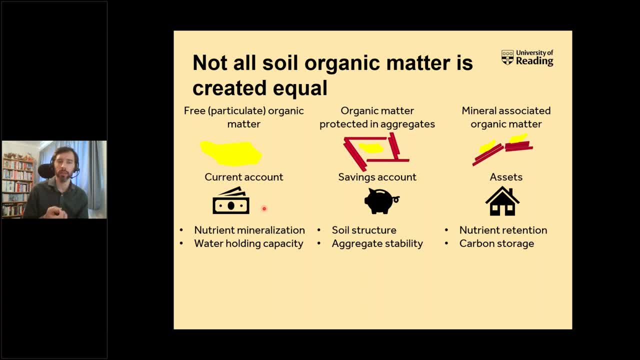 available to plants. And then there's the organic matter that's produced by the soil. So when it's decomposed, those nutrients are released and made available to plants. It also helps with the soils to hold water as well. The organic matter that's protected aggregates. this helps the 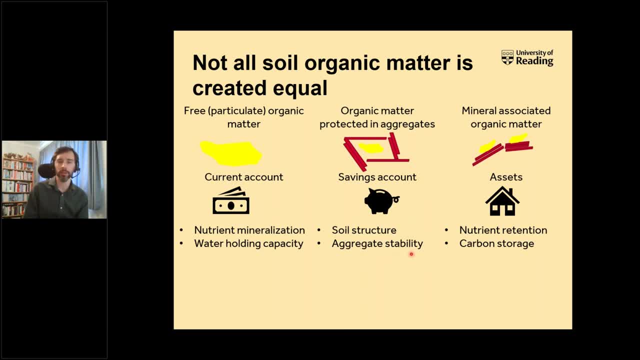 structure of the soil by generating those stable aggregates And the mineral associated organic matter. this is where you get that kind of ability for that soil to retain nutrients and prevent them from leaching, And also it's our long term carbon store in soils as well. 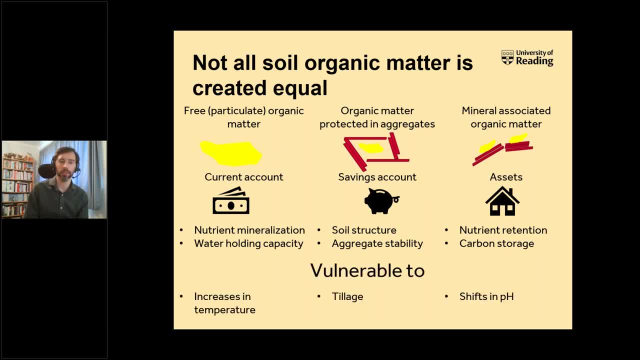 But all three of these pools are vulnerable to greater or lesser extent. Probably the most vulnerable is the free particulate organic matter, but it might be vulnerable to increases in temperature, because we know that at higher temperatures we tend to get higher rates of decomposition. Our aggregate protected pool is vulnerable to tillage, So if we plow, 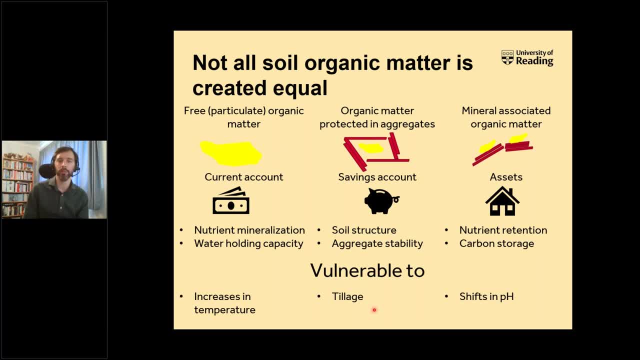 up our soils and disrupt those aggregates, then we're making that carbon available to the soil microbial community that can metabolize it. The mineral associated organic matter is much more stable than the other two pools but it might be vulnerable, for example, to things like shifts in pH. So if the pH of the soil changes, then that means that. 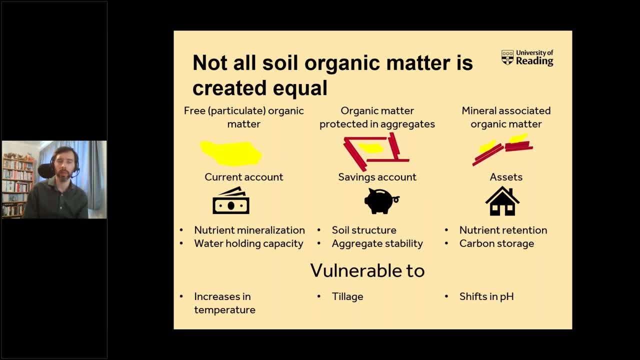 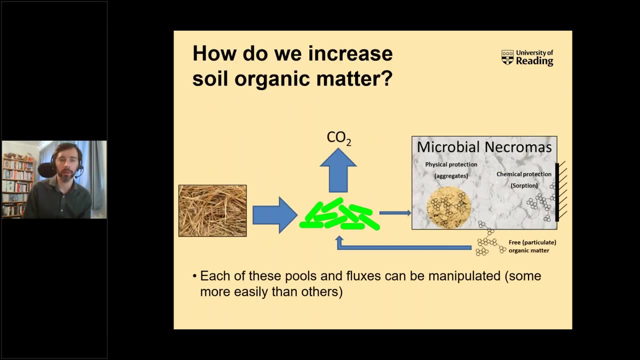 the soil, organic matter can become desorbed from the surface. So, for example, land use changes that require large shifts in pH might result in release of some of that stable mineral associated organic matter. But one of the key steps that I want to talk about, 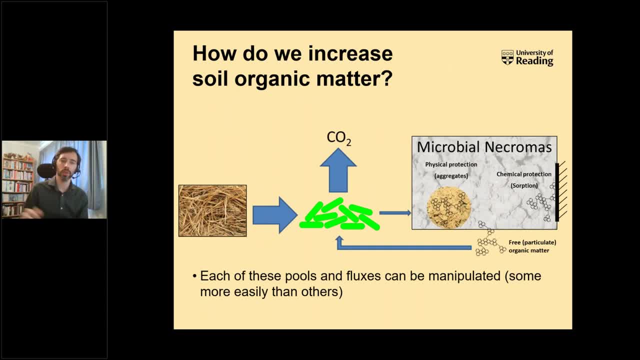 in the process by which organic matter becomes soil. organic matter is what happens to this initial resource as it enters into this soil microbial community. Ultimately, what we can do is we want to be able to increase the amount of that carbon that comes into that microbial community and decrease the amount that leaves the system. 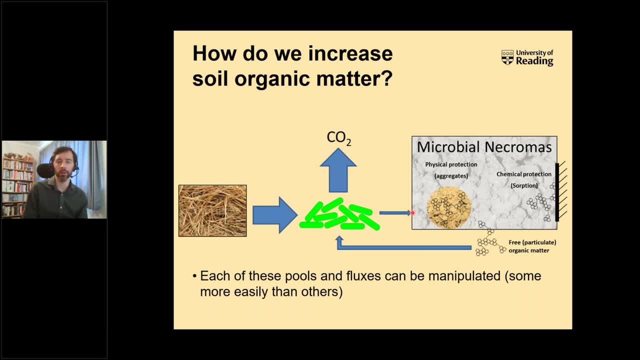 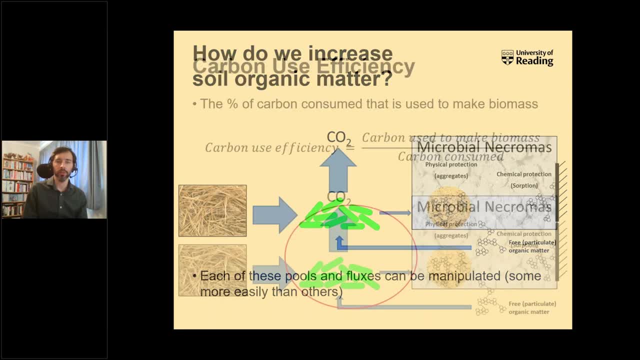 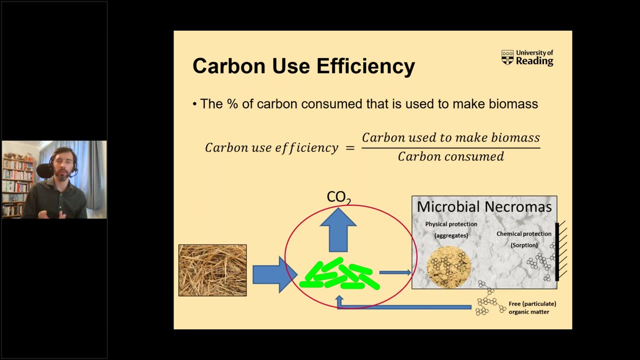 as carbon dioxide, Because that means we get more dead microbes that then can become that microbial necromass which ultimately becomes our long term carbon. So that's the And the concept of this process whereby microbes might either use that carbon to make their microbial biomass or what we refer to as anabolism, against using that carbon to respire and use for energy and respiring it as carbon dioxide, which is what we refer to as catabolism. 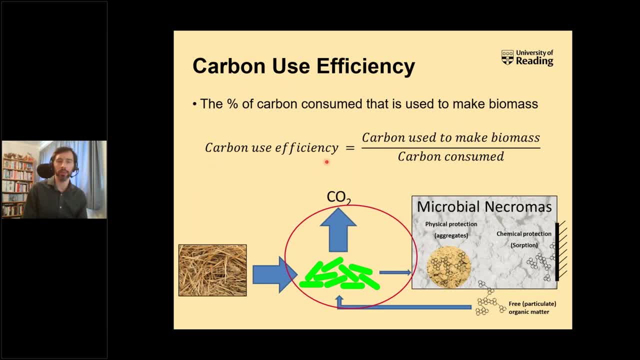 So this can be kind of embodied within this idea of carbon use efficiency. So this is the amount of carbon that the microbes use to build their biomass divided by the total amount that's being consumed, So the total amount that's entering into the soil. 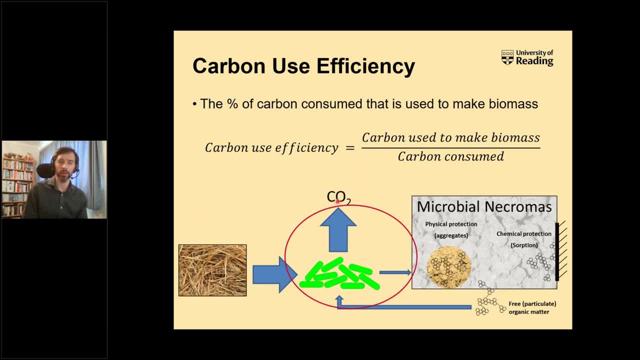 So a soil with a high carbon use efficiency means we've got a larger soil microbial biomass And ultimately we hope that it becomes a high soil microbial necromass which can become our long term stable carbon storage. So ultimately, what I'll talk about today is ways in which we can increase soil carbon use efficiency. 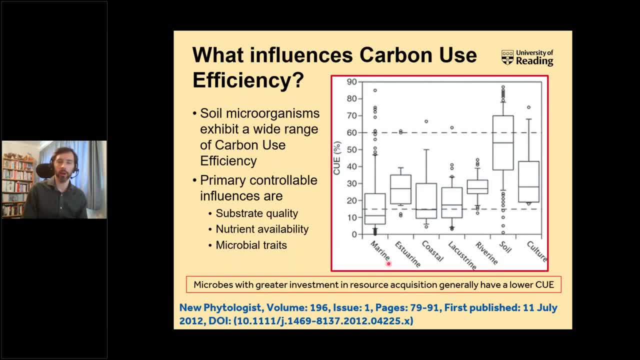 And it's worth mentioning that, compared to a few other different environments- so marine, estuarine, coastal environments- that the soil carbon use efficiency is much higher than we see and we observe in other types of environments. But at the same time, the range of carbon use efficiencies that our soil microbial communities can exhibit is also quite high. 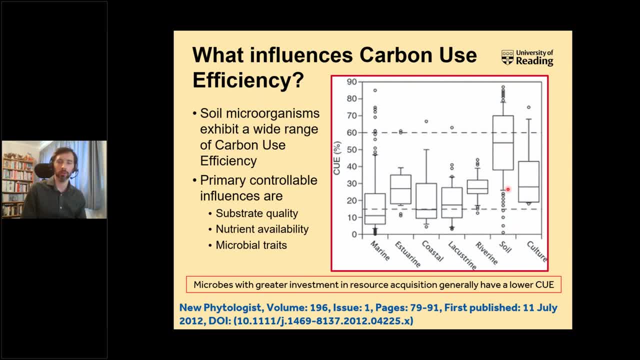 And so we might have some soils that are operating at the very low end of this range, where most of that carbon is being released as CO2.. And we may have other soils that are operating with a very high carbon use efficiency, where most of that carbon is going into the microbial biomass. 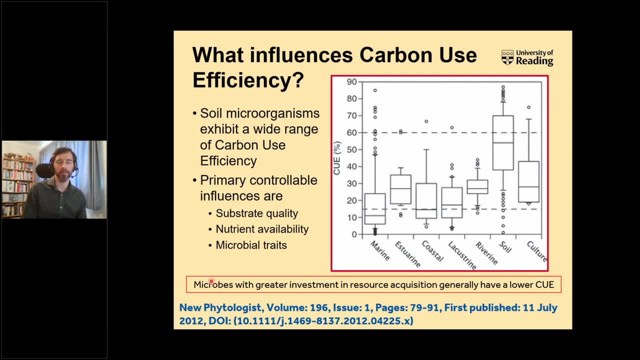 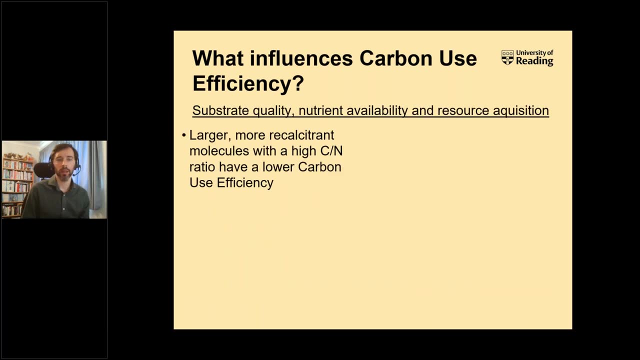 And some of the key things that can influence the extent to which we have a high carbon use efficiency is the investment of those microbes need to make in acquiring carbon, their resources. So the amount of the type of carbon amendment that we add into the soil, the quality of that substrate and the nutrients that are available and dictate the carbon use efficiency. 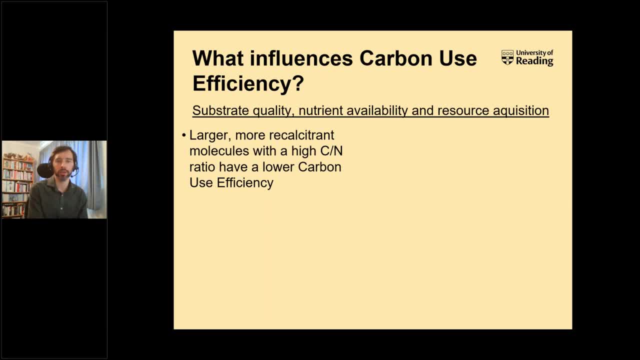 So larger, more recalcitrant molecules with a high carbon to nitrogen ratio. they typically have a low carbon use efficiency And these kind of remind me of the squirrel from the Ice Age movies. So if you've not seen the movie, the squirrel kind of pops up every 10 or 15 minutes and he 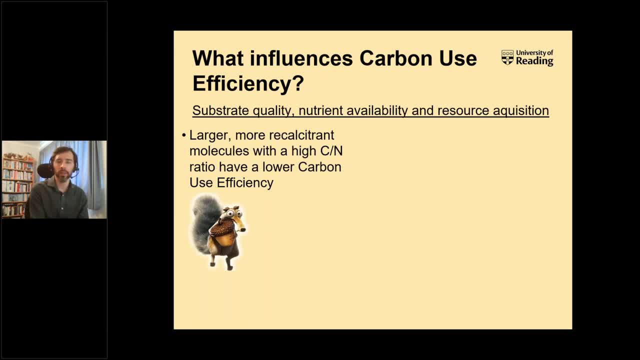 spends lots of energy chasing around this acorn And by the end of the movie you kind of wonder whether the squirrel has spent more of its energy trying to get this acorn than it would actually gain from actually eating it, And by way of analogy this might represent sort of straw. 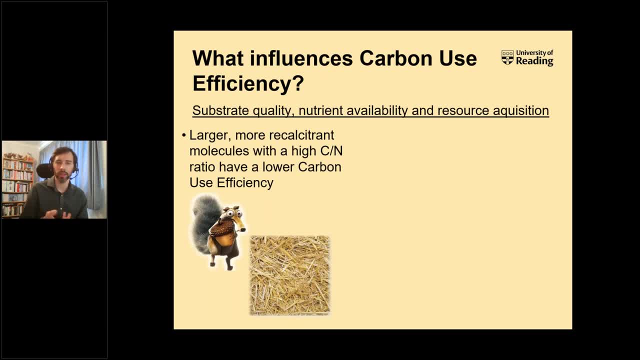 or something with a high lignin content, not very much nitrogen. It would be very difficult for the soil microorganisms to break down. On the flip side, we could have low molecular weight compounds, so simple sugars that have perhaps a high C to N ratio and a much higher carbon use efficiency. 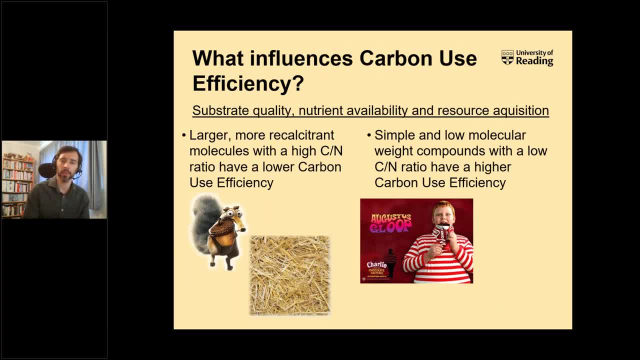 So, again using an analogy, this might be similar to Augustus Gloop from the Charlie and the Chocolate Factory movie. So Augustus Gloop is a big fan of chocolates and sweets and things, And, of course, he's very fat as well as a result. So this is kind of what we want, our 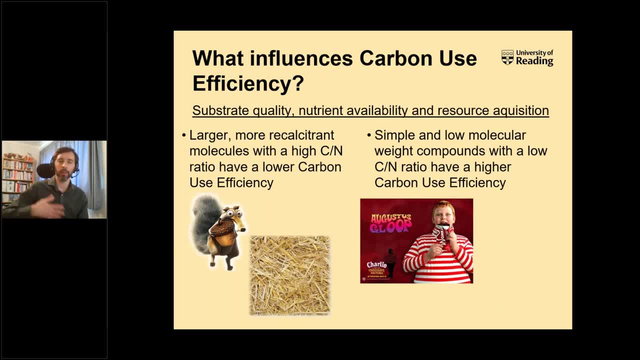 microbial community to do. So this is kind of what we want our microbial community to do. We want them to be fat, We want them to become larger, We want them to use that carbon to build biomass, And these simple sugars might be coming from plant root exudates. 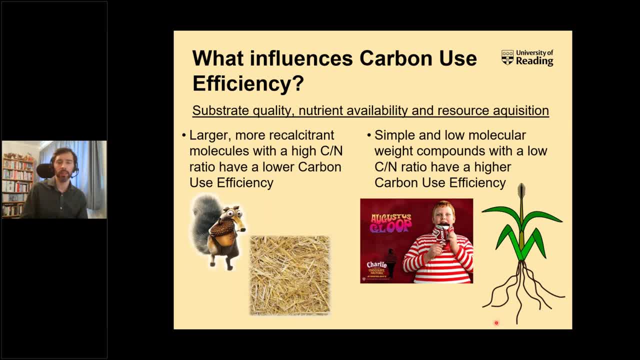 for example, these sugars that the plant root is pumping into the soil, Of course the plant root exudates typically don't contain much nitrogen, So nitrogen is also required by that community in order to build soil organic matter. So what we add into the soil can have. 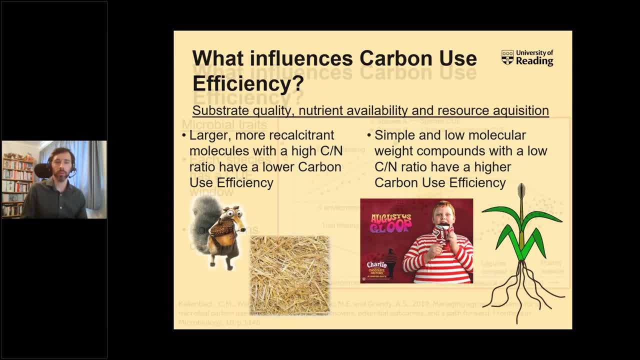 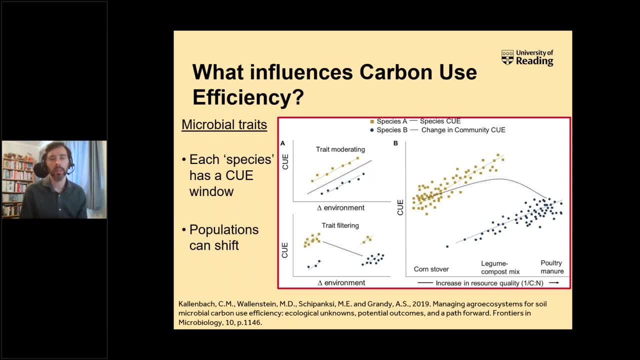 an influence on the carbon use efficiency. I also want to share this concept here, which is published by Cynthia Kallenbach and co-authors two years ago now. It's a really neat paper basically explains that each individual microbial community will have its own. 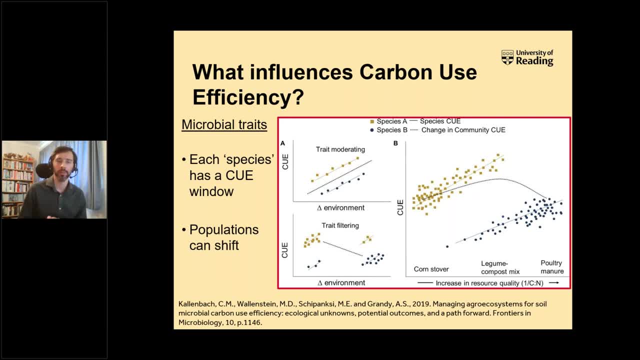 window of carbon use efficiency that it operates within, And so you can change the environmental conditions in order to change the carbon use efficiency of the pre-existing microbial community, But at the same time, you can also add in the carbon use efficiency of the pre-existing 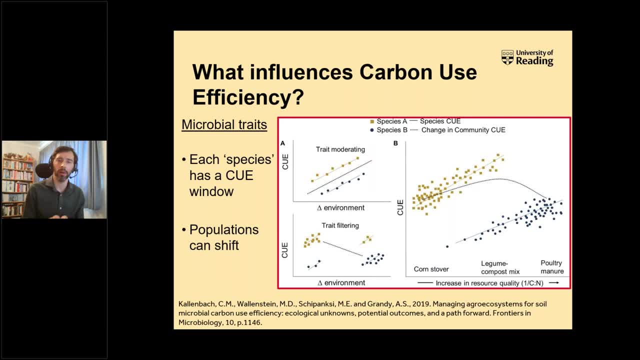 microbial community. So at the same time, you can also shift the population of the microbial community that you have in your soil to one that might operate at a higher carbon use efficiency. And what was proposed in this paper, I should say the data that's being presented on 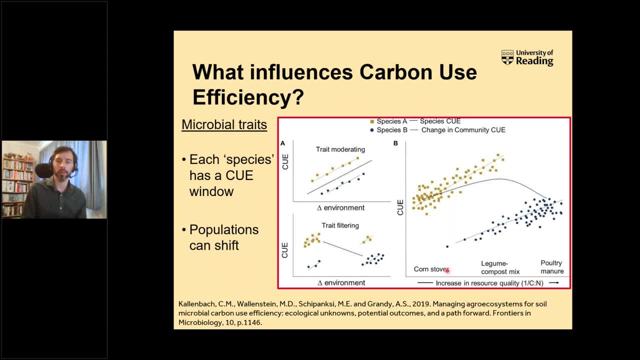 the screen here is that you might be able to. on one side you could have sort of a high C2N ratio material or a low C2N ratio material, But there are benefits to be gained by mixing high and low C2N ratio material, So you can have a high C2N ratio material and a low C2N ratio material. 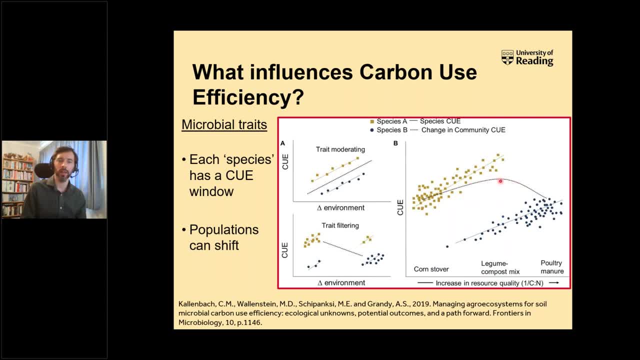 So you can have a high C2N ratio material and a low C2N ratio material in order to optimize the carbon use efficiency and ultimately result in more carbon going into the microbial biomass and a little bit less leaving the system as carbon dioxide. We tried this in a field experiment, So 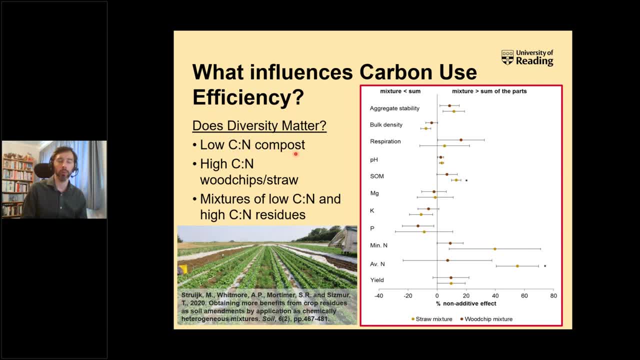 we mixed some low C2N ratio compost and vegetable waste compost with some high C2N ratio materials like wood chips or straws, And we did an experiment where we looked at the mixture versus the sum of the parts and then we plotted, we measured a whole bunch of different things. 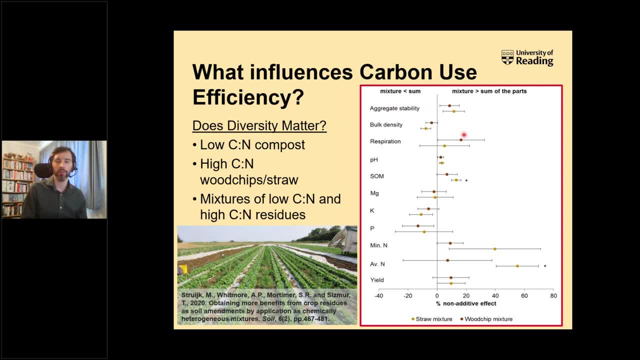 and plot them on this graph, And if they appear on the right-hand side of the graph, this means that the mixture is greater than the sum of the parts. If they appear on the left-hand side of this graph, then the mixture is less than the sum of the parts. And one of the things we measured was: 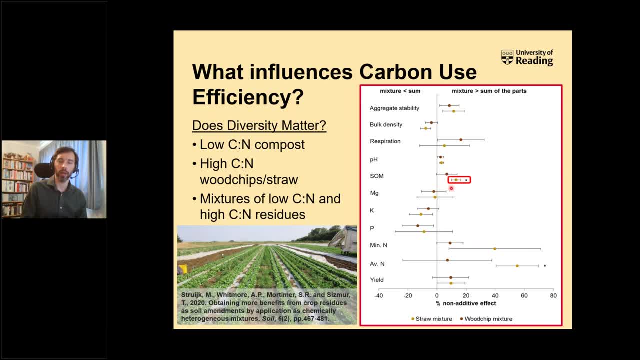 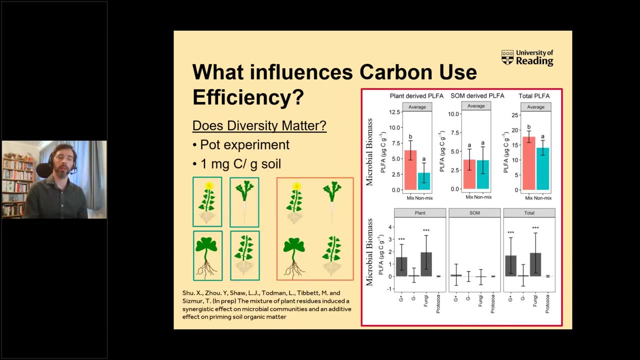 soil organic matter and we found that the soil organic matter that we built in that soil was greater than the sum of the parts when we applied that high and low C2N ratio material ratio mixture together. So this cost us thinking a bit more about diversity and whether it matters. 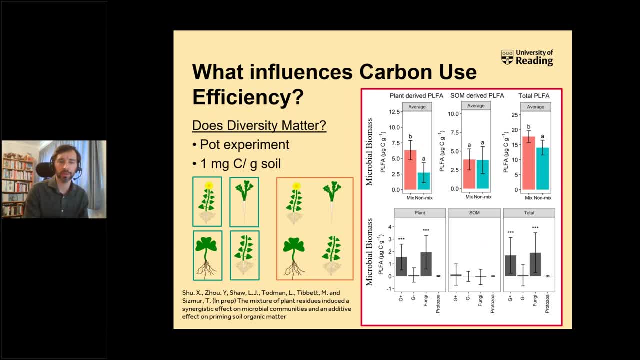 whether we add a more diverse mixture of substrates into our soils, and here we did a much more controlled experiment in the laboratory. so it was a very small pot scale experiment, and to every treatment we added the same amount of carbon, and we either added that carbon in the 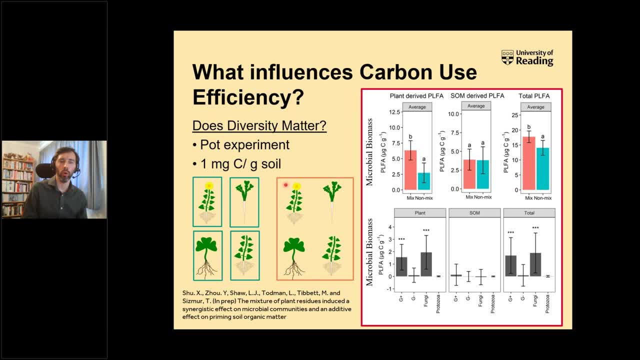 form of the residues of a single crop or we added that carbon in the residues of a mixture of four different crops. and the crops we used here were typical cover crops that farmers might grow in between two cash crops in a cereal rotation. So we have sunflower, we have radish, we have clover. 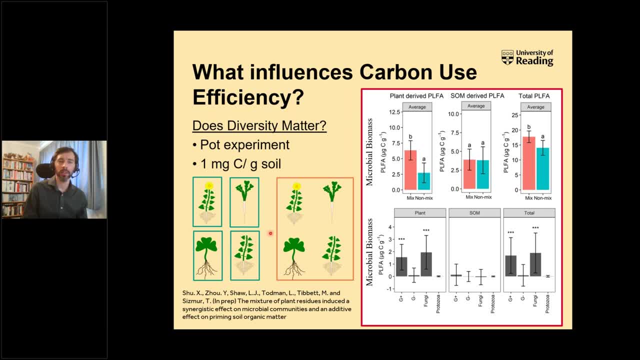 and we have buckwheat, and so we then compared, similar to the last experiment. we compared what happened to a you have. you have add the mixture versus the average of the sum of the parts, and what we were looking at was the soil, microbial biomass, which we measured using a technique referred to as PLFA or phospholipid fatty. 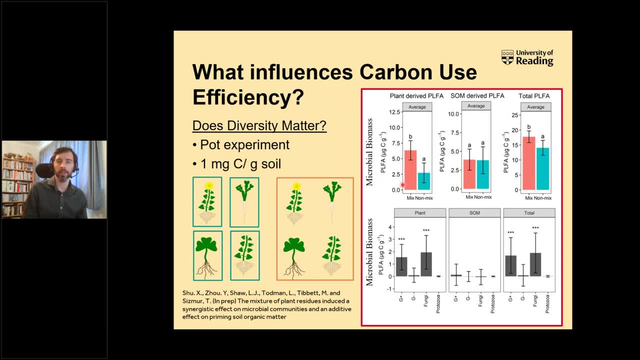 acid analysis and here we can see our orange or pink bar is higher than our turquoise bar, and what this means is that when we mix those four residues together we get more of that plant derived carbon going into the microbial biomass. we also looked at the extent to which adding these plant residues primed the decomposition of the soil organic matter that was already in the soil and we saw no difference. 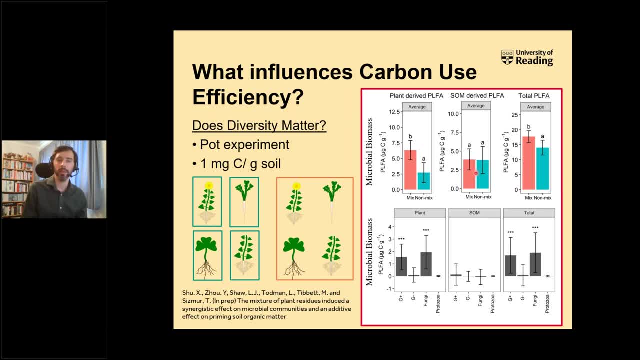 whereas all these treatments did prime soil organic matter, we didn't see any difference between the mixture and the sum of the parts. We also looked at which microbial communities were responsible for this difference that we observed here, and we saw the gram-positive bacteria and our fungi and the 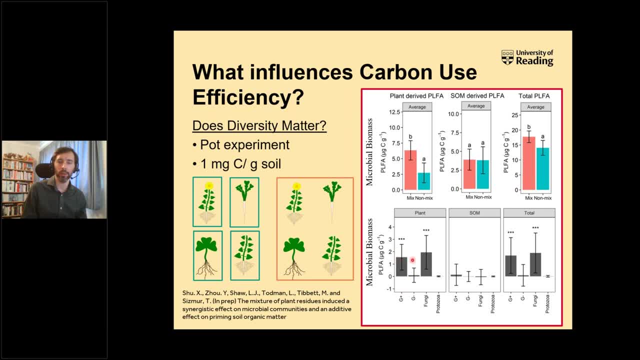 bacteria alsomışed out a mixture, or a group as well, which we then saw was high in the lamp средn chapters as that which was used, depending on how many of the biomes that we trying to try to get to from where we are today with the five that we created before we decided on those, there was a delay between minimum harmonics, known as lack of concentration. 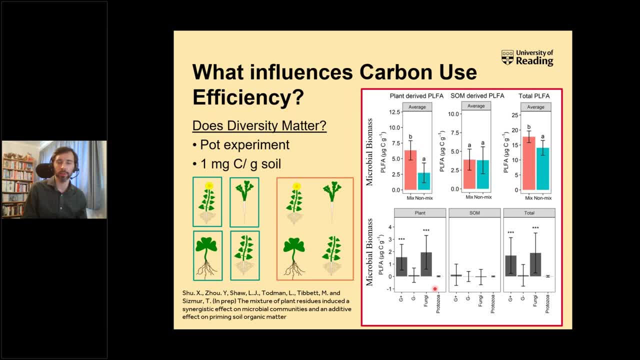 and our fungi communities were primarily responsible for this difference, and this is consistent with the idea that our gram positive microbes and our fungal communities are a little bit. they tend to have a higher carbon use efficiency anyway. so we think to some extent that there are some benefits to be obtained by mixing plant residues as they go into. 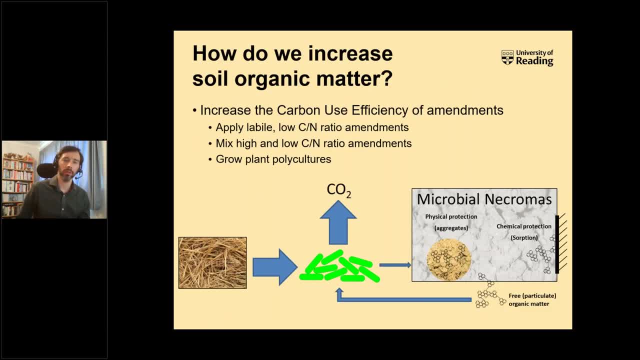 the soil. So just to summarize on carbon use efficiency. so there's kind of three primary techniques that I'm introducing that we might be able to use to increase the carbon use efficiency of our amendments. We can either apply a sort of label- low C to N ratio amendments- so those 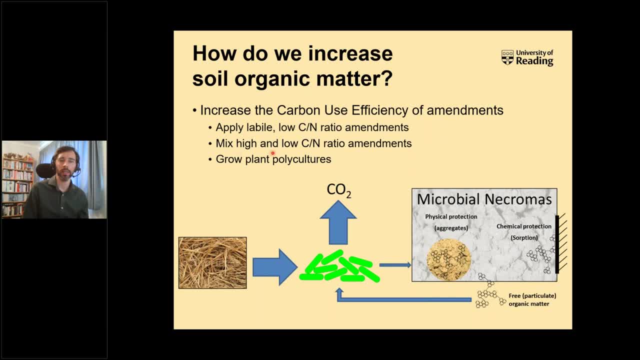 simple sugars that feed things like Augustus gloop, or we can mix some of our high and low C to N ratio amendments, accepting the fact that you know we have these amendments like straw. perhaps we can still use them and also there seems to be some benefits by growing plants. 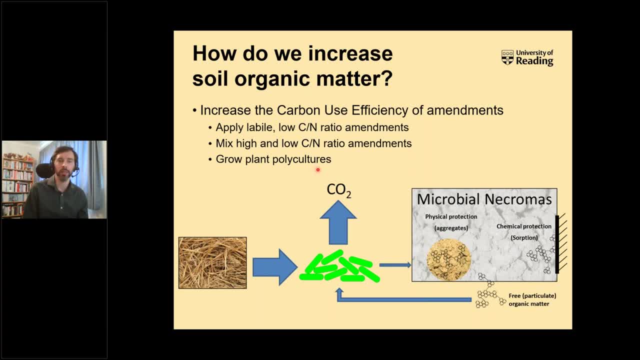 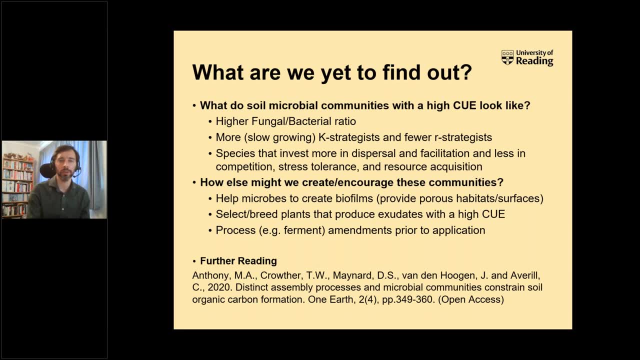 in polycultures, so we've got a mixture of diverse substrates entering into our soil. So just to end by thinking a little bit more about the future and to sort of share some ideas, I'll be very happy for people to use the chat box to let them know what they. 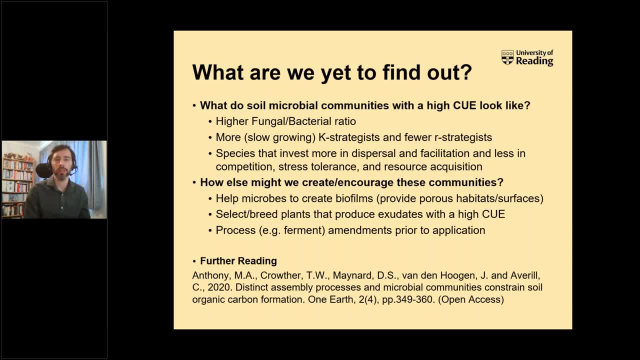 think of these sort of ideas, but I'm starting to think about. so what are these microbial communities that have got a high carbon use efficiency? look like Ryan Jackson. We think they probably have a higher fungal to bacterial ratio. usually they tend to have more sort of what we call K strategists. So these are 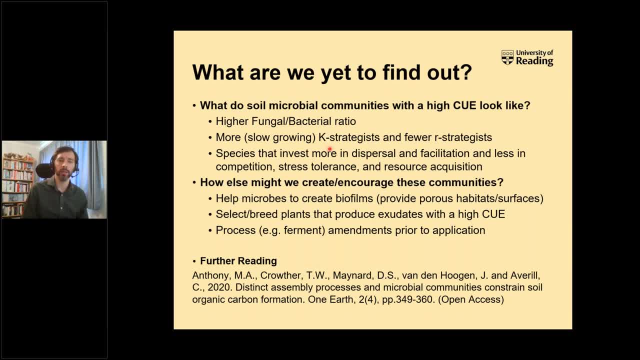 a little bit like using the analogy of the hare and the tortoise, So that the tortoise is more like a K strategists and an R strategist would be more like the hare. So they're slightly slower growing And, just broadly speaking, we're looking for species the invest more of their energy in the 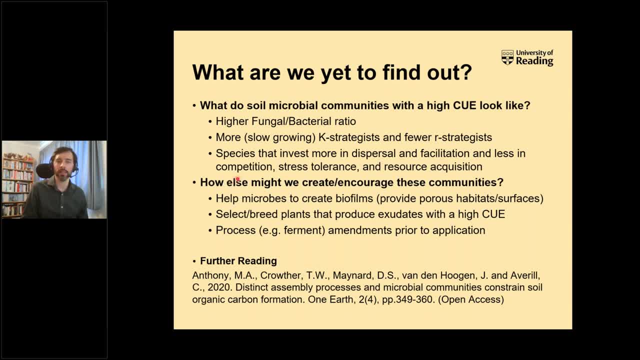 dispersal or facilitation, cooperation a little bit less in competition or tolerating stress or acquiring their resources. So we could think about things like how we promote biofilm formation in soils. Do we provide sort of porous materials, perhaps biochar, zeolites, that kind of thing? 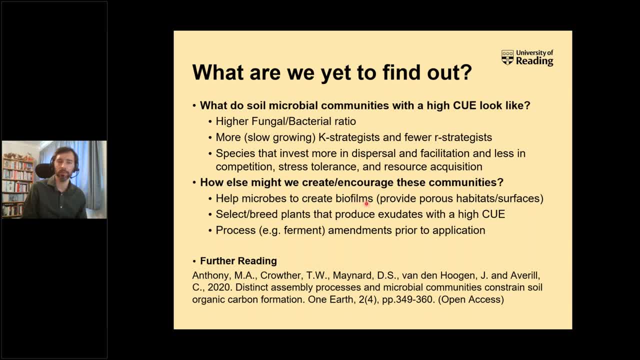 surfaces which might help the creation of biofilms, because we know that biofilms have a slightly higher carbon use efficiency. Do we need to select or breed plant communities that might produce these exudates with a high carbon use efficiency, Or are there things that we could? 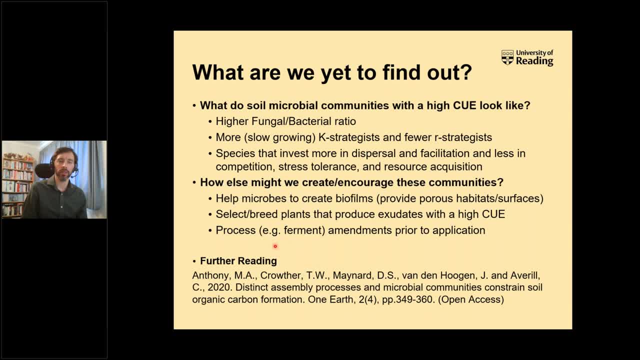 sort of do to the soil amendments before we add them to the soil. So, for example, might we ferment them or do some other process in which we convert that carbon into a form that might then have a higher carbon use efficiency. And I guess, just to shout out that if you're looking to sort of 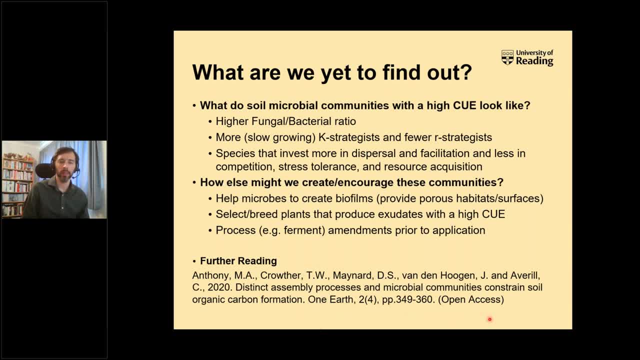 things. a bit of further reading on this as well. this is a fantastic paper published almost a year ago now by some authors in Switzerland, Which kind of talks through this idea about how we can use soil microbial communities, And there's a few ideas, including some on this slide, that have come from this paper as well. 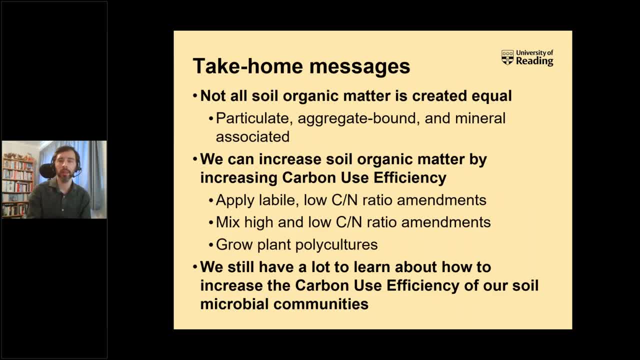 So I'll just end with my take home messages. So again that there's three different key types of organic matter in the soil. They're particulate bound, aggregate bound and mineral associated. There are strategies that we can adopt to increase the carbon use efficiency. 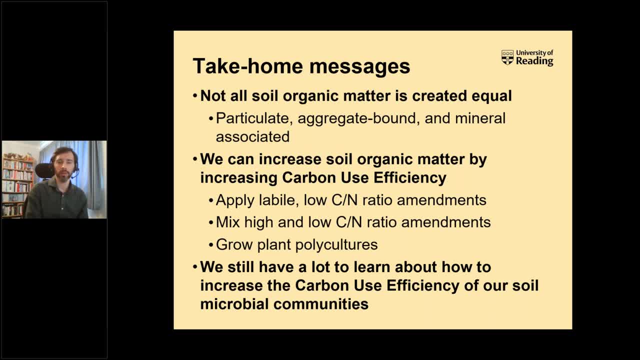 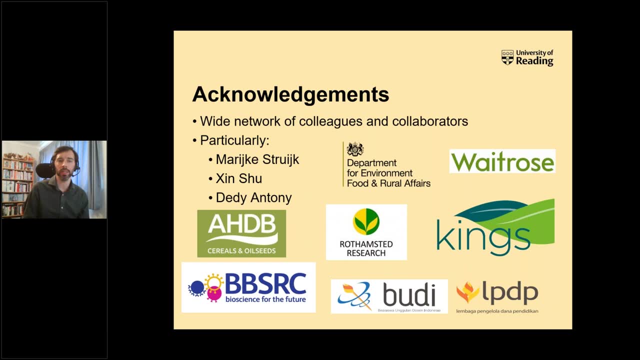 of the soil organic matter That we add into our soil. And, of course, there's a lot more that we can learn, and there's a lot more research that needs to be done in the future in order to advance our understanding, And so with that, I'll just share my acknowledgements, particularly Marijke Strauch. 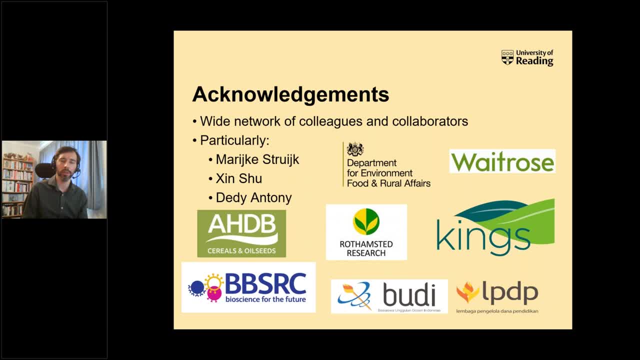 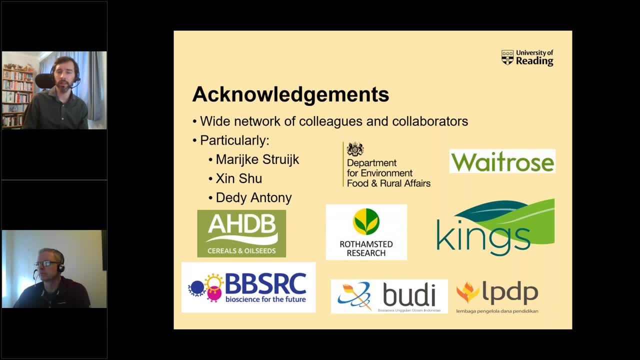 Xin Xu and Deddy Anthony, but also a whole bunch of funders and organisations that we work with, Of course. I will thank you for listening, And now I'll hand over To Bruce, who I think will will introduce Julian for his presentation. 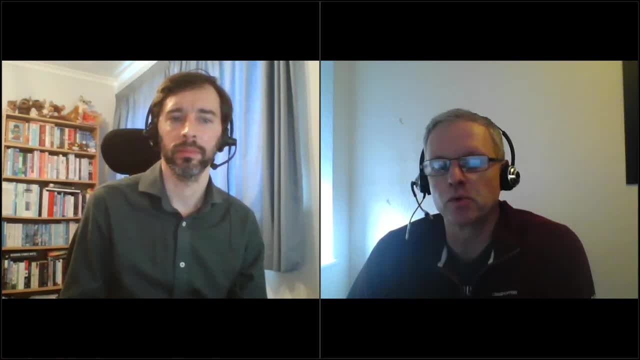 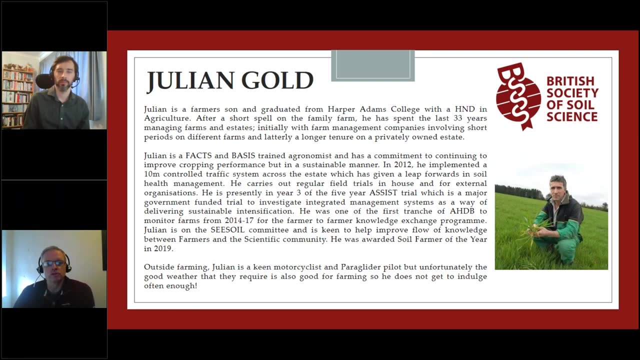 Yeah, thank you very much, Tom. That was excellent, And just a reminder: we will be taking questions for both speakers at the end of the session. So our next speaker is Julian Gold. Julian is a farmer's son and graduated from Harpurcut Adams College with an HND in agriculture. 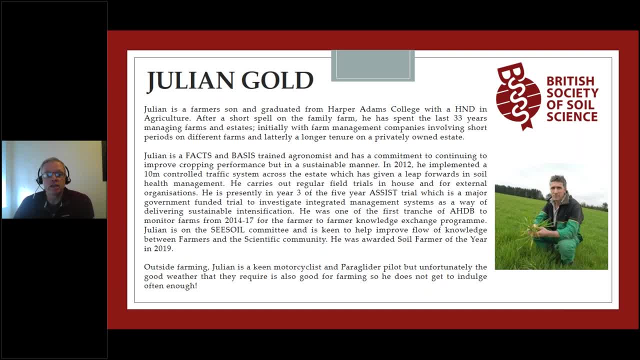 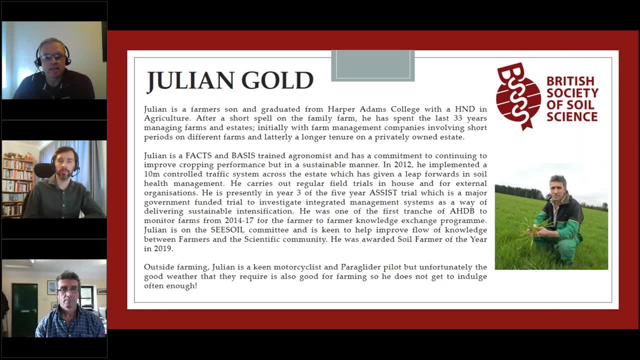 After a short spell on the family farm. he spent the last 33 years managing farms and estates, initially with a farm management company, And he's been working for a number of companies, involving short periods on different farms and, latterly, a longer tenure on a privately owned estate. 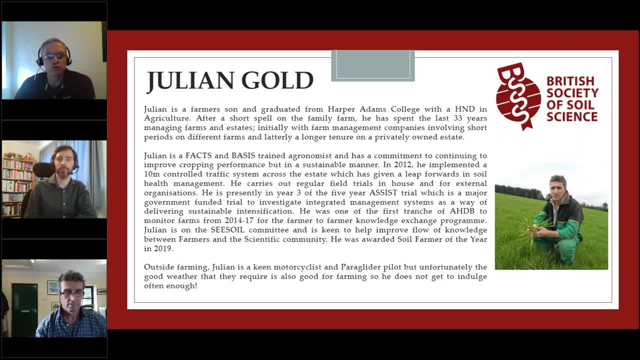 Julian is a facts and basis trained agronomist and has a commitment to continuing to improve cropping performance, but in a sustainable manner. In 2012,, he implemented a 10 metre controlled traffic system across the estate, which has given a leap forward in soil health management. 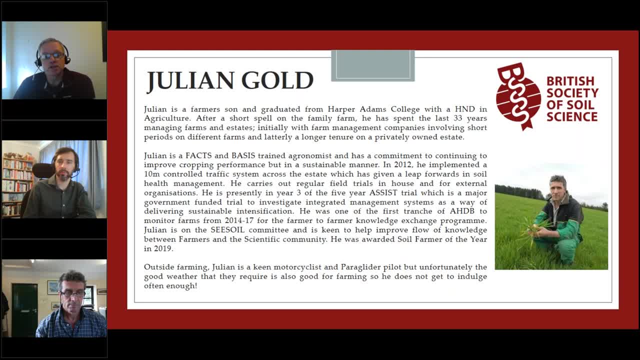 He carries out regular field trials, in-house and for external organisations, And he is presently- And he is presently in charge of a five year ASSIST trial, which is a major government funded trial to investigate integrated management systems as a way of delivering sustainable intensification. 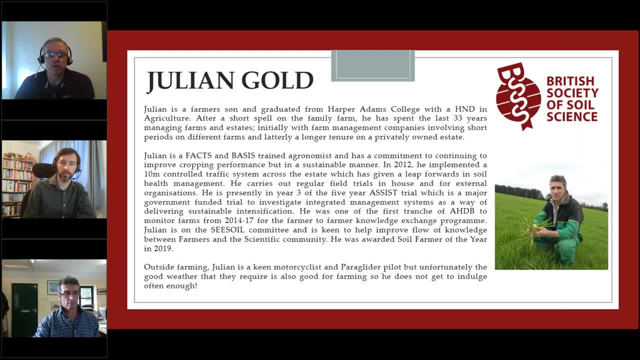 He was one of the first tranche of AHDB to monitor farms from 2014 to 2017, for the farmer to farmer knowledge exchange programme. Julian is on the Sea Soil Committee and is keen to help improve the flow of knowledge between farmers and the scientific community And he was awarded the Soil. 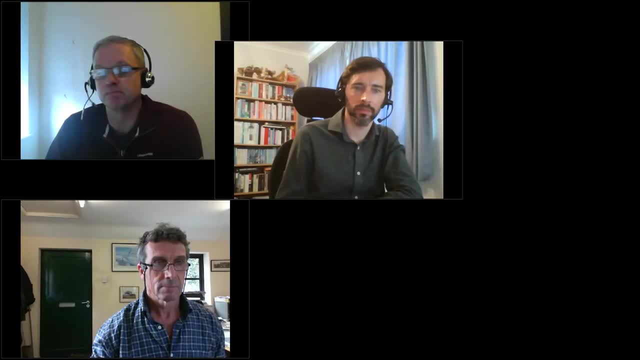 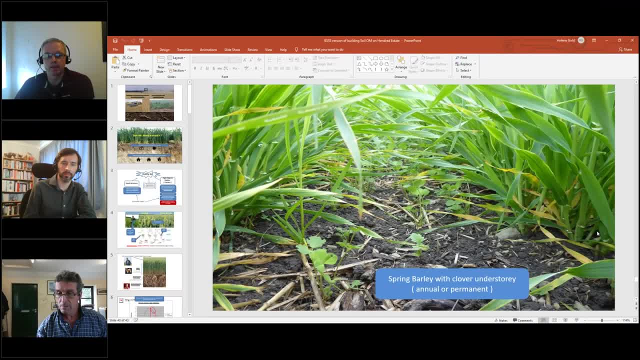 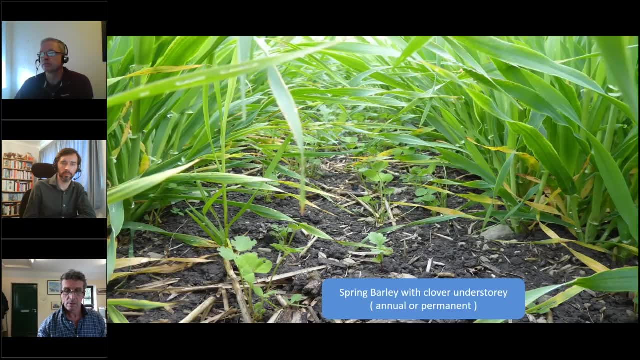 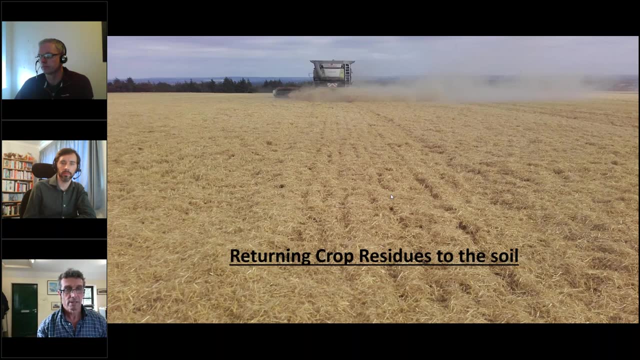 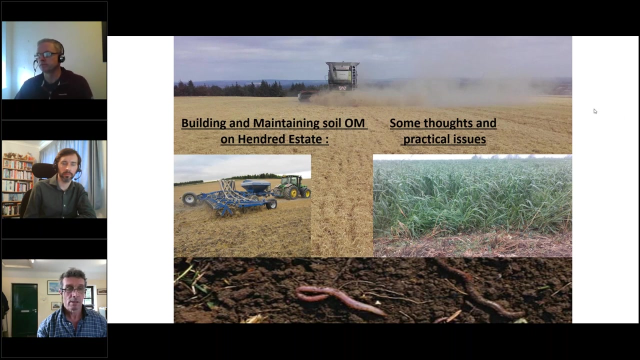 Thanks, Bruce, Just trying to show my screen. right. I cannot see or see anything on the screen other than my presentation. Right? I cannot see or see anything from the screen other than my presentation, So I will leave that for you to have a look at it next time. See you then. 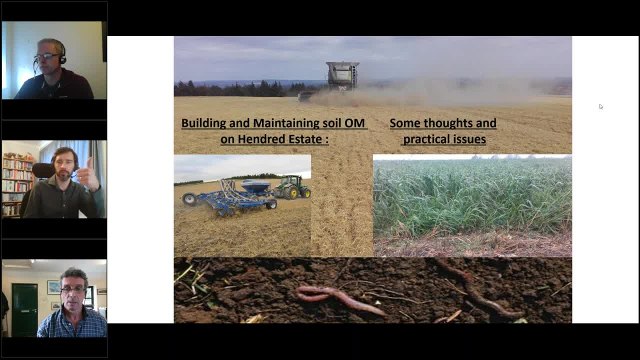 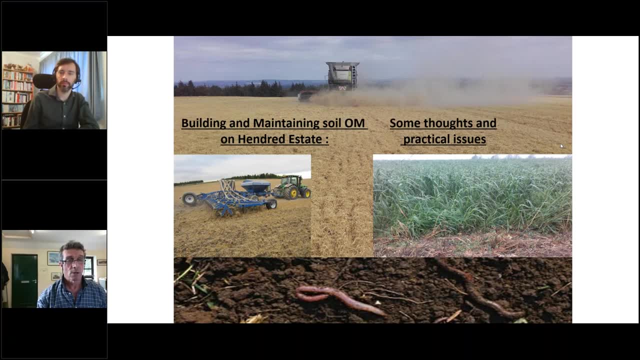 hopefully everybody can hear me. could somebody just confirm? yeah, we can hear you, julian. okay, thank you. um right, yes, um building on tom's talk, i really just want to whiz through and show you what this building and maintaining soil organic matter looks like on farm in practice and some of the 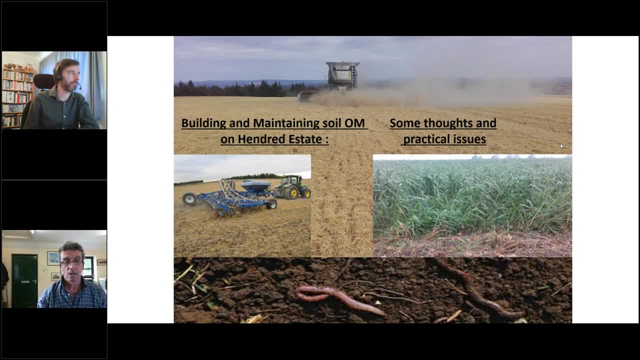 problems. now this is a very um site specific talk because unhindered estate. we haven't got any organic amendments really going into the system. we're predominantly a cropping farm with a few sheep on permanent pasture and cover crops um, so we're trying to build organic matter without 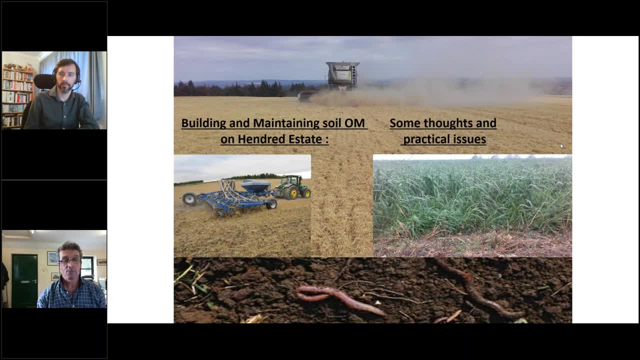 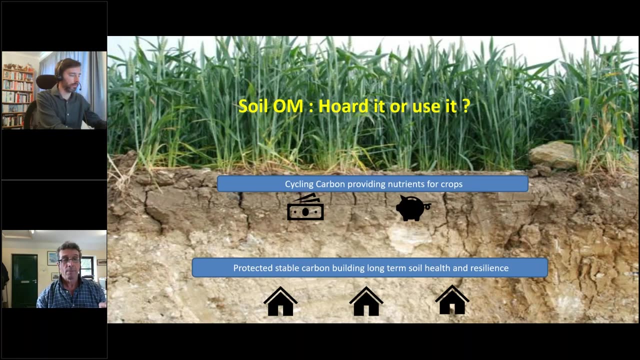 rotational lays and without a lot of organic amendments like fm and compost, um, so that makes it a little bit harder for us, but we are achieving quite good results. hopefully you'll see um just thinking about as a farmer, just thinking about soil organic matter, um, that's obviously the big dilemma: soil organic matter. do you hoard it or use it? well, as a farmer. 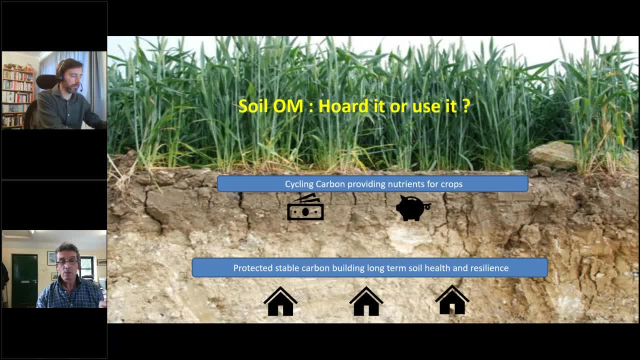 i want to build soil, organic matter in my soil for long-term soil health and um sustainability. but i also want organic matter to be cycling in the system i want. i don't want to be relying on all my nutrition from artificial fertilizer sources. i want to be mineralizing organic. 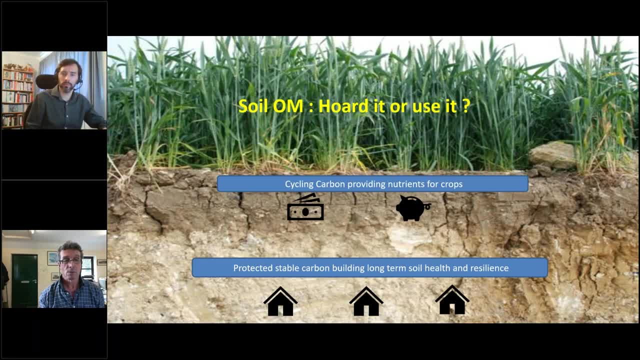 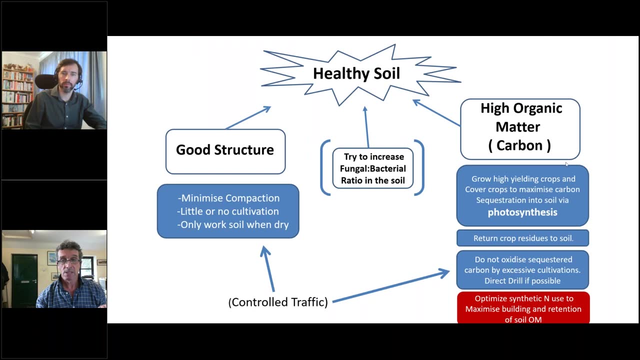 matter and providing nutrients for crops. um, to obviously help with our economic yield of crops, is trying to achieve this happy medium of building soil organic matter but also using soil organic matter. um, and you'll see how we try to do that as i go through the talk. um, this is a slide that i will. 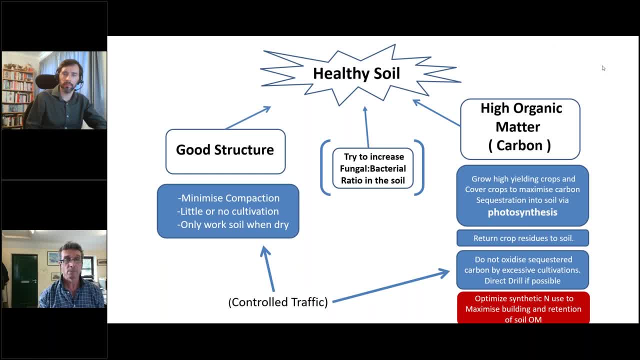 um, go back to a few times. basically this: this summarizes, on hundred estate, how we're trying to build healthy soil in our system and obviously healthy soil. you're talking good structure on the left hand side and you're talking about building soil, organic matter, on the right hand side, and I've got my little techniques in the blue and red boxes that I'm 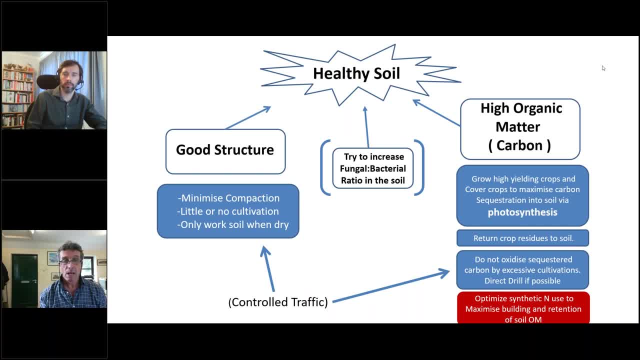 going to talk about through the talk as to how we're achieving this. Also, in the middle you'll see the sort of little one in brackets trying to increase the fungal bacterial ratio in the soil. I'm very aware that in intensively farmed systems such as ours, it's our dominant. 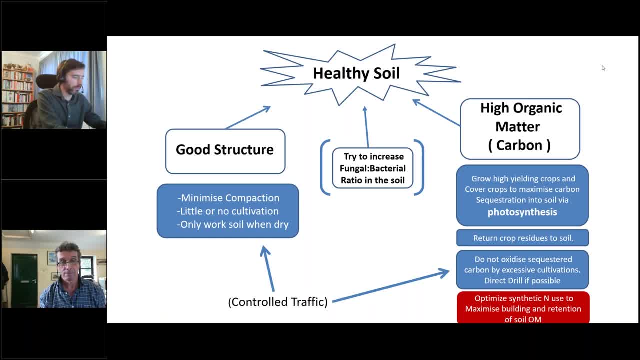 ratio is bacterial to fungal is higher bacterial than fungal. but obviously we've got lots of advantages with increasing fungal numbers. You've got things like mycorrhizal associations that are improving crop yields. you've got things like better carbon use efficiency, as Tom pointed out. 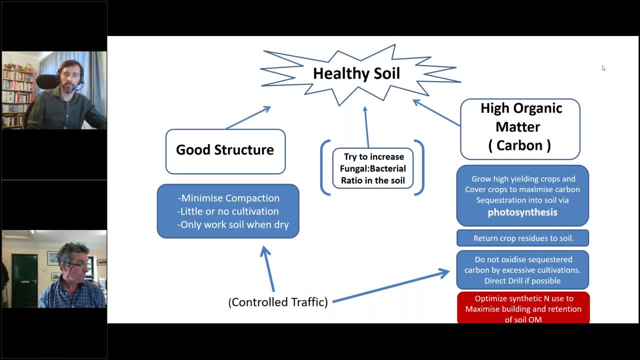 with fungi rather than bacteria and you've got just the fungi's ability to improve soil aggregation and carbon stability in the soil. So I've got that one in the middle in brackets. it's one that I've constantly got in the back of my mind. I think in practice it's very difficult to influence easily. 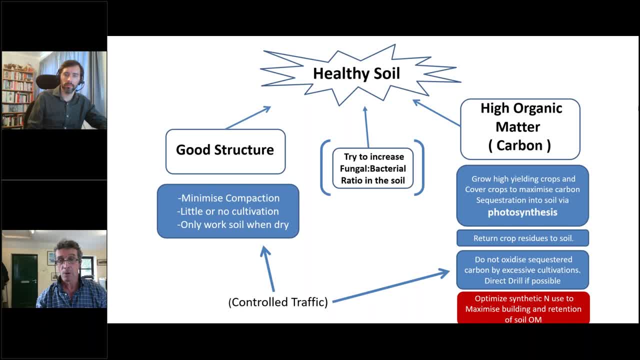 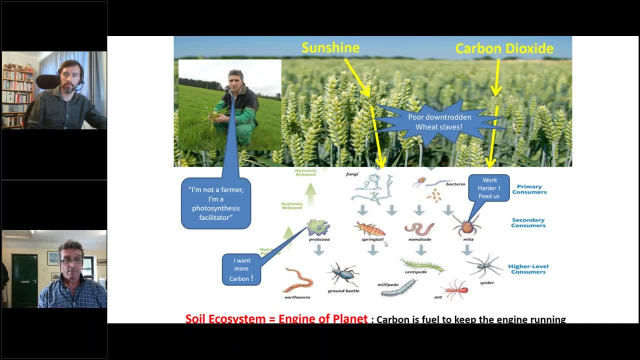 in a commercial farming situation. but just going through all the others one by one, starting with the photosynthesis on the right hand side, Yeah, I really see myself not as a farmer, I see myself as a photosynthesis facilitator and a bit like a method actor. I like to sort of get myself in role. 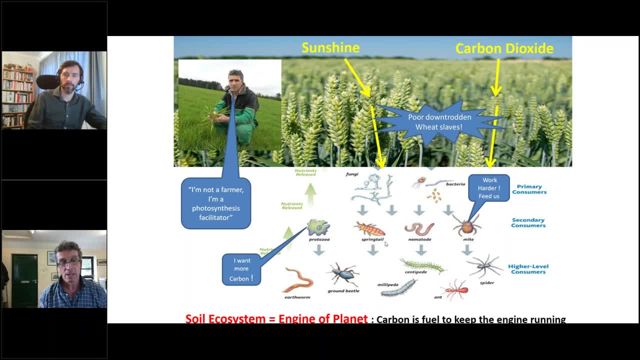 for what I'm trying to achieve on the farm and I like to sort of try and imagine this sort of fantasy of this intelligent soil ecosystem and it's sort of employing crops to grow in it to feed the carbon and it's employing me to tend the crops and for my work they're sort of giving me. 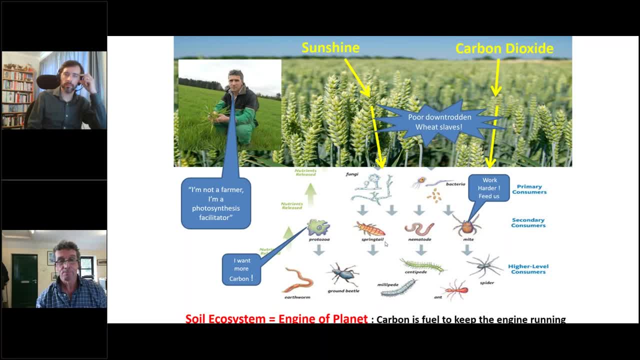 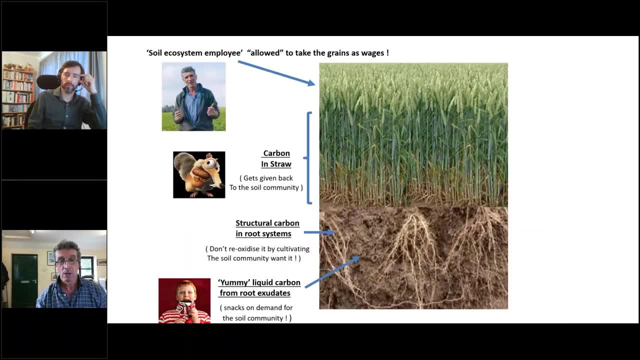 the grains as a reward for tending the crops, and that's my sort of fairly naive way of just sort of thinking about how I'm managing my farm and my cropping system. looked at another way, and using some of Tom's analogies with the squirrel and Augustus Gloop, you've got the crops. 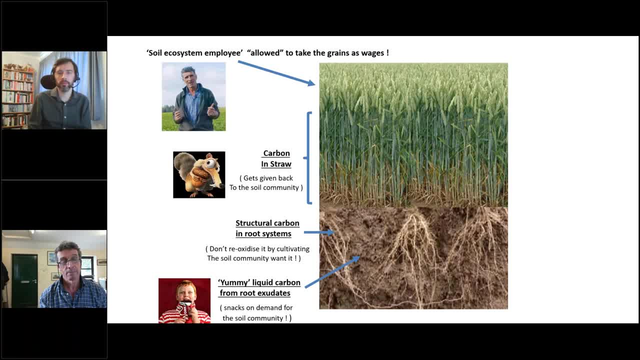 growing in the soil system there, with me concentrating on feeding the soil system and, I think that, in the grains as wages. and I think that it's interesting that the actual end result, by me concentrating on working for the soil system rather than working for a big crop yield, it gives me a big crop yield as a side, as a sort of result of getting a healthy. 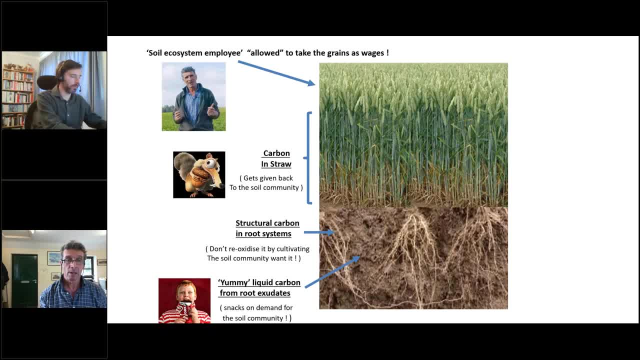 soil and working on looking after the soil ecosystem, I naturally get big yields of grains, and so it's just a sort of different emphasis, but it gives you a better- the same or better end results as concentrating on maximizing your crop yield, and then you've got everything going back into the 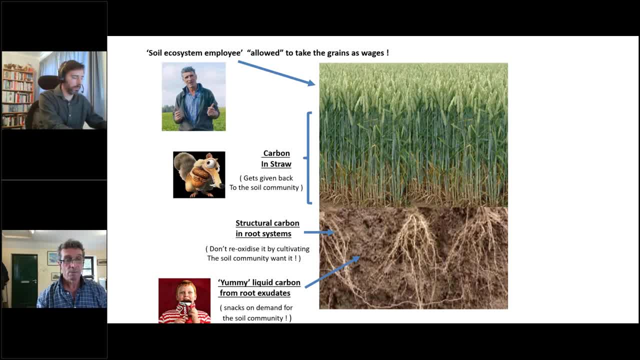 soil system, the carbon in the straw, and you'll see through the talk that this is a big issue. that's caused us a lot of problems over the years, because I've sort of had this fixation on this lower carbon use efficiency straw and getting that back into the soil system, whereas I'm over the 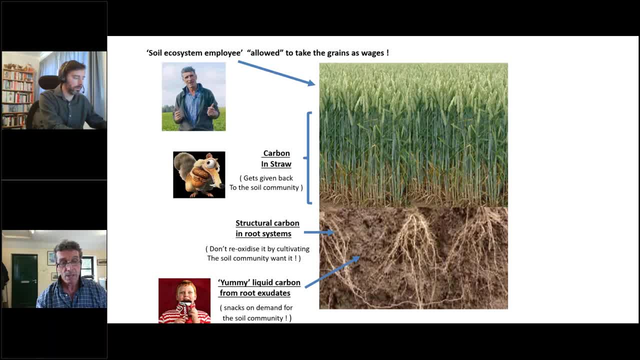 years I think I've probably been detrimental to some of the better carbon use efficiency things like root exudates going into the soil system. so I've been concentrating on maximizing your crop yield going into the system. but we'll see that as we go through. so, thinking about photosynthesis: 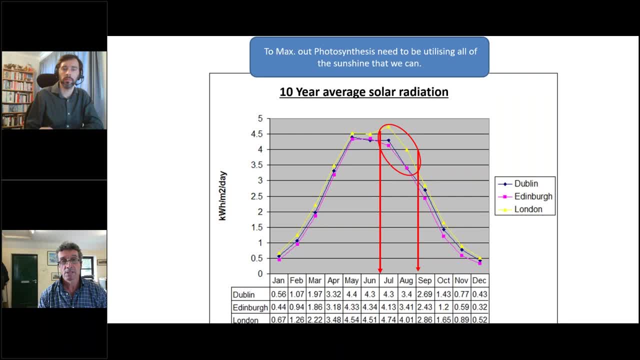 obviously one of the main things with photosynthesis. we need to max out our utilization of solar radiation and that's just a graph, sort of teaching grandma to suck eggs. more sunshine in the summer and obviously with our cash crops as sunshine's building through the spring and early. 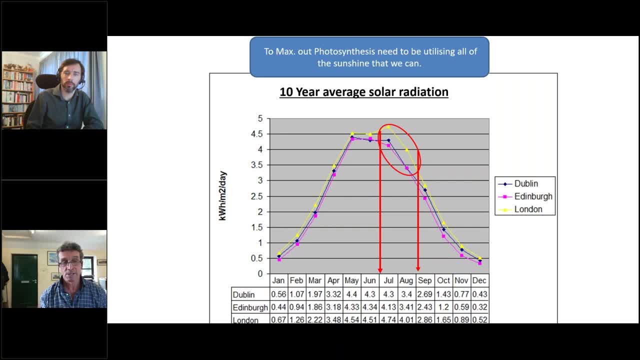 summer we're maximizing the photosynthesis and the biomass yield by judicious use of inputs and and trying to grow the crops as efficiently as we can to maximize the yield and maximize root exudates and crop biomass going back into the system. but then I think the trick is in building. 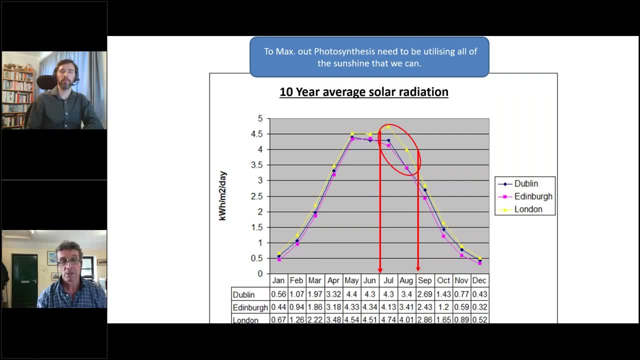 soil organic matter is sort of sneaking in those extra bits of photosynthesis. the big thing for me is this July, August, early September period where you've got a lot of solar radiation and traditionally you've got no crops in the system. so this is where you cover crops and you catch crops. 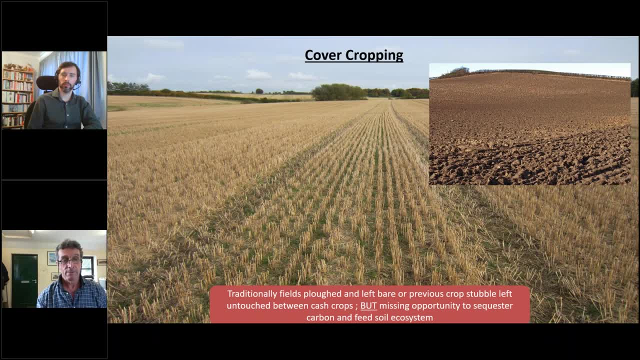 traditionally. obviously that's the sort of scenario you might have seen on farms between summer harvested crops and spring planted crops: bare stumbles, even plowed cultivated fields with nothing growing on them. bit of a missed trick, really, missing out on photosynthesis. so we're putting cover crops in the wherever we can and the other thing 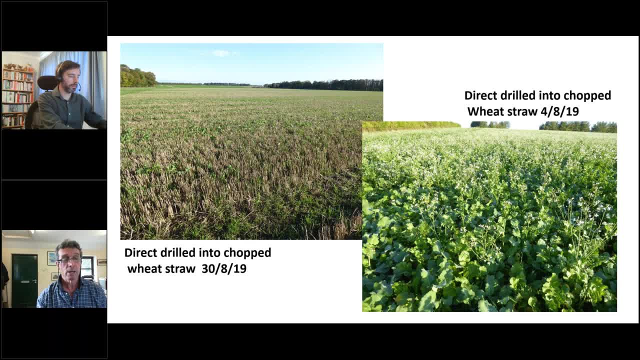 about cover crops and thinking about maxing out that solar radiation. we need to get the crops in the ground and growing that. the drill needs to be in the field with combined harvest. so absolutely, as is- this is last year- the field on the right drilled on the 4th of August on the left. 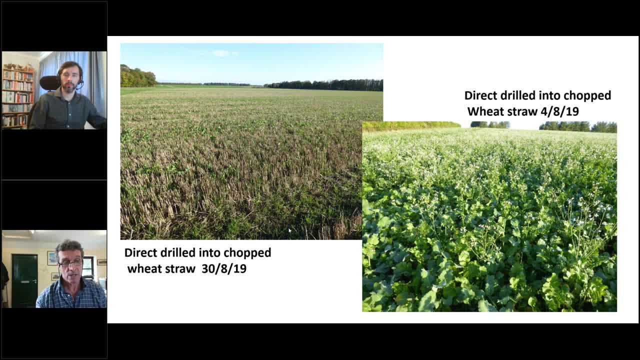 exactly the same mix on the same soil type into the same scenario of chopped wheat straw drilled nearly a month later, their photos in October: the one on the right is up around your waist and the one on the left is barely taller than the stubble. so again, if we're going to utilize this radiation in the summer, we 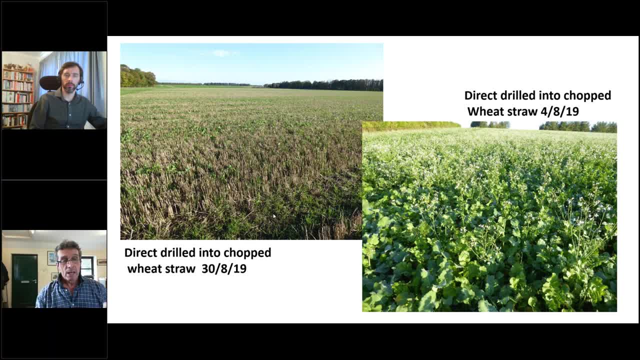 need to get the crops in the ground and growing. the other thing obviously is catch crops between, as well as cover crops between summer harvested crops and spring crops- is whether you can get catch crops in between summer harvested crops and winter planted crops, and people try to do this in the UK. we don't. 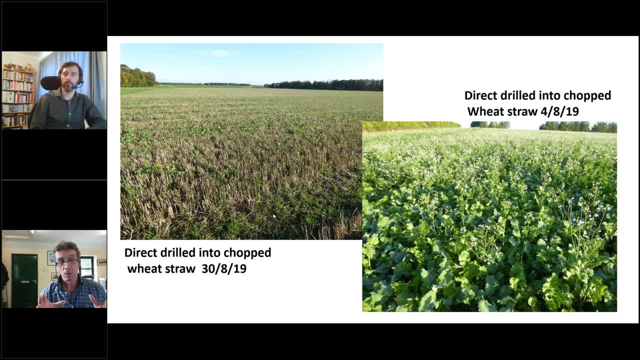 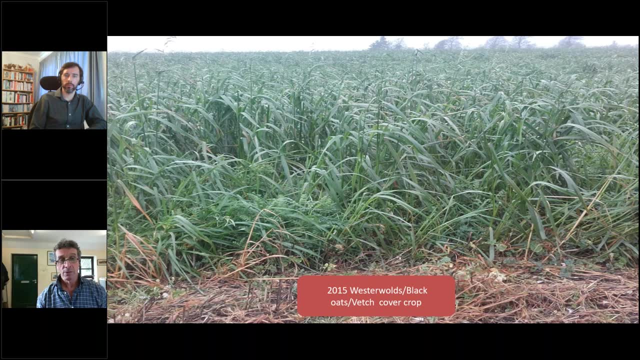 try. I think it's too difficult. people put mustard crops in and quick growing crops and try and get a bit of a crop growing there, but I think it's quite. it's quite difficult. in UK conditions, cover crops early on tended to be about two or three things in the mix high. 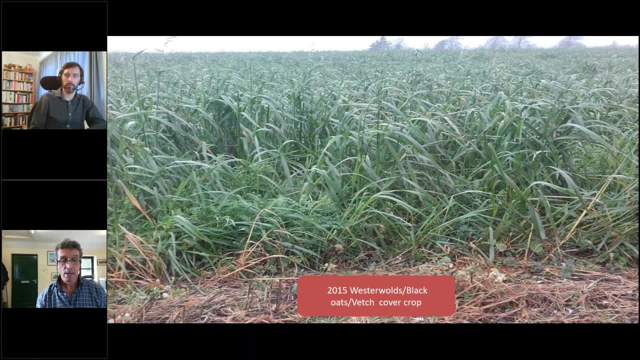 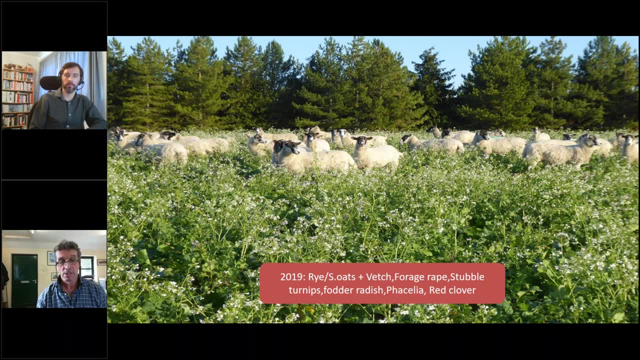 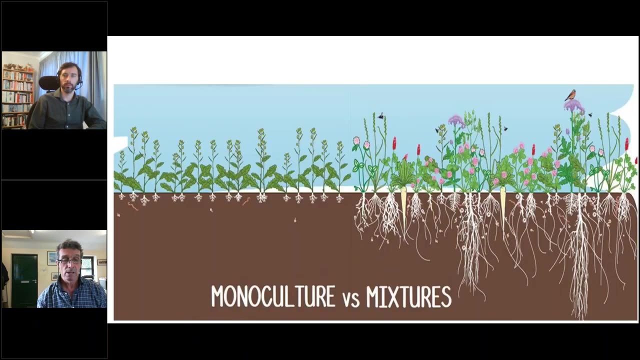 biomass. we're aiming for high biomass cover crops and then grazing them off with sheep. as the years have gone by, the mix has got more diverse and more intricate. that was last year's cover crop mix. many more legumes in the mix now and less cereals. various reasons for mixtures. we want a diversity of root. 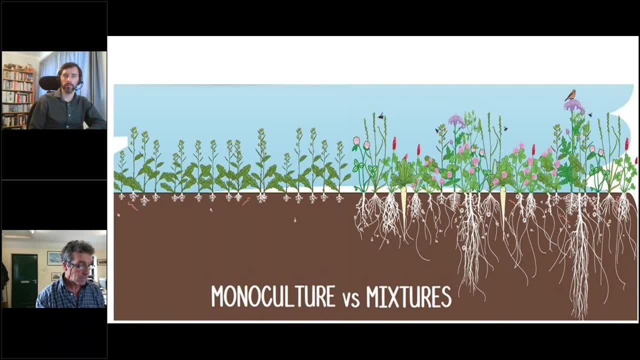 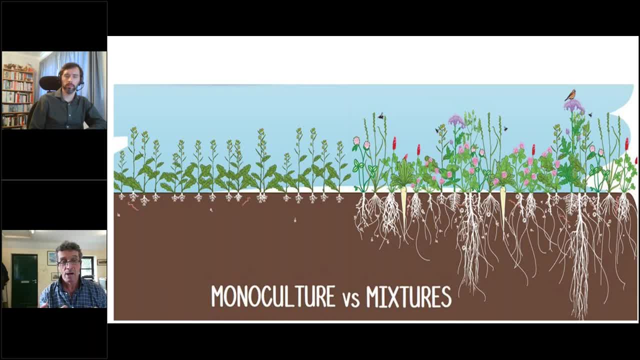 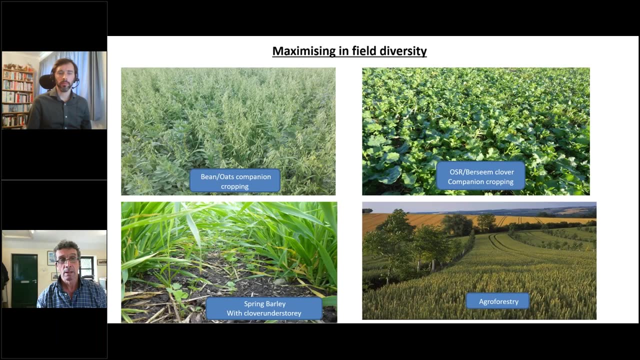 carbon use efficiency from different plants. you've also got a range of CN ratio is, which has given you again a better community carbon use efficiency. it's all about getting diversity into the rhizosphere and into the soil and and just while we have mixtures and diversity without cash crops as well, our 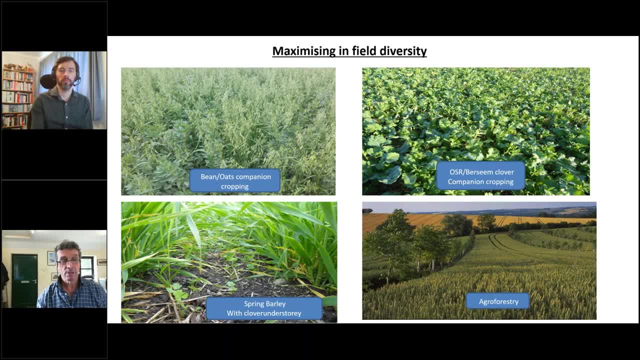 we're playing around trying to maximize infield diversity and for the last few years, been playing around with understories, companion cropping and the ultimate one in the bottom right hand corner, agroforestry, is one of my pet favorites that we haven't really got around to um doing yet, but 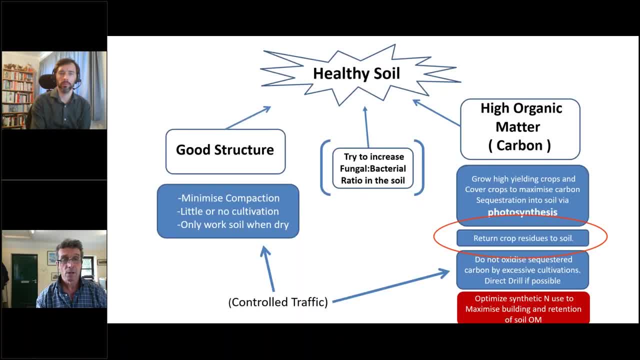 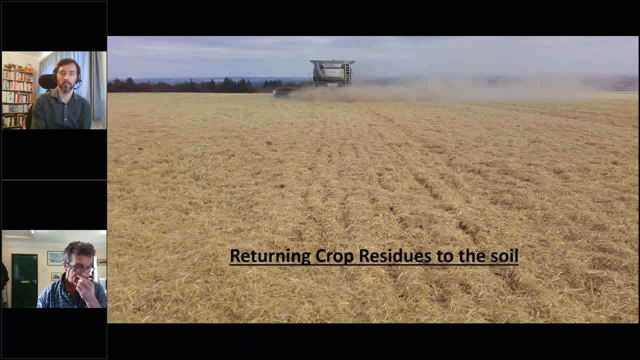 hopefully sometime in the future. um right, going back to my main slide now to talk a bit about returning crop residues. this is something that over the years- um, as i alluded to, alluded to earlier on- i've spent a lot of effort on returning crop residues and i think a lot of it has been. 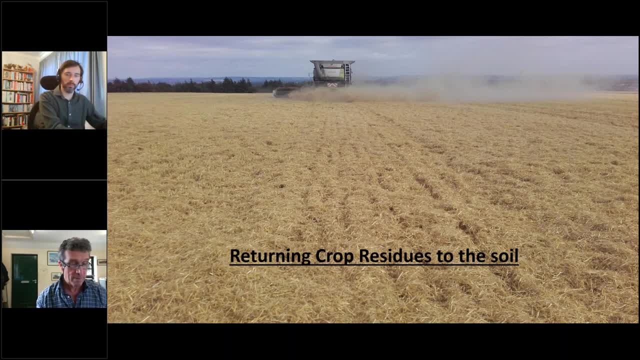 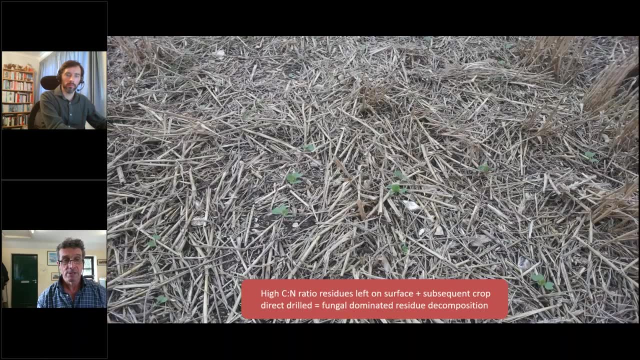 sort of misguided really, and a lot of the problems it's caused us have probably been detrimental to our overall soil organic matter improvements. um, obviously you've got a range of outcomes with um crop residues sort of one extreme here is your high cn ratio cereal straws left on the 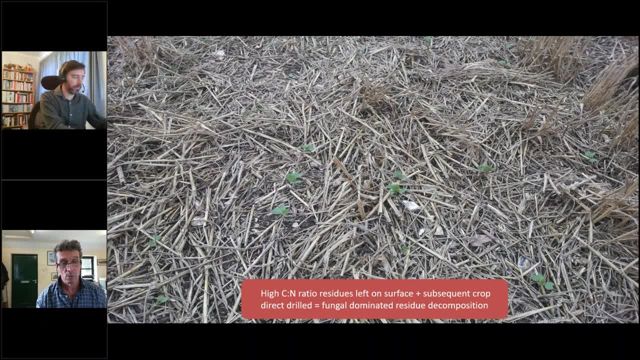 surface um and your subsequent crop. we've got all seed right there direct drilled. you've got a fungal dominated residue decomposition there and these are the situations where obviously you're hoping the net end result into the soil system is the best but that gives us the most problems in. 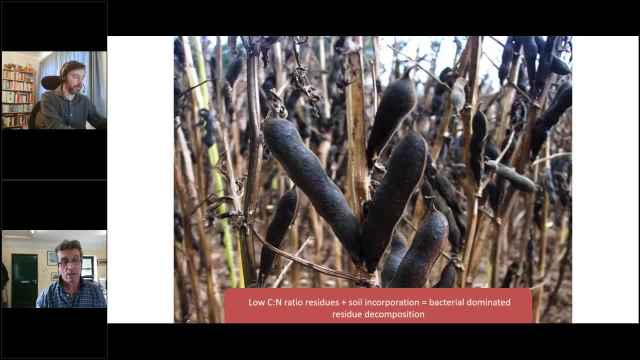 establishing following crops. you've got another extreme here where you might grow low cn ratio crops like beans and, to an extent, or seed rape, if their residues are soil incorporated. you're sort of tending to towards bacterial dominated residue decomposition, um not quite so beneficial in the soil system, um we find that these also grape and bean residues. 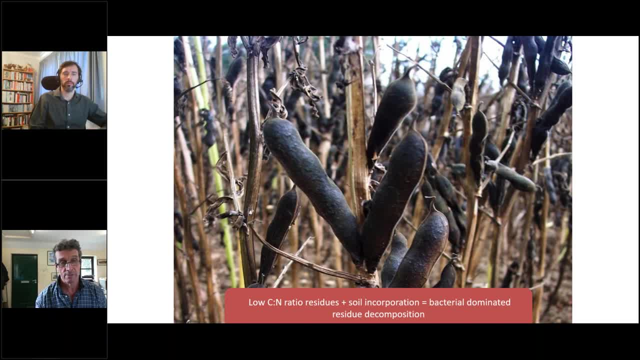 in practice we don't incorporate them. they're just left on the surface, the same as the cereal ones, but they give us very little um problem with establishing following crops, mainly because it's cereals after them. um, but obviously you haven't got problems with residue decomposition. 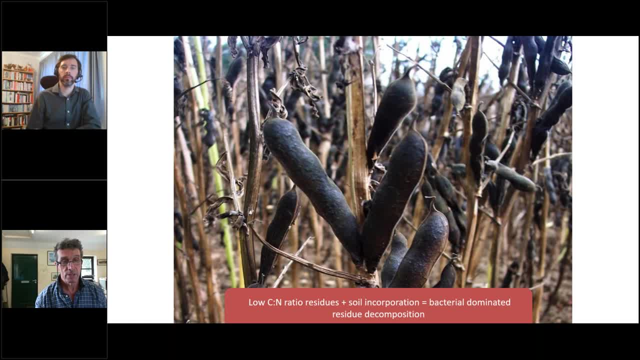 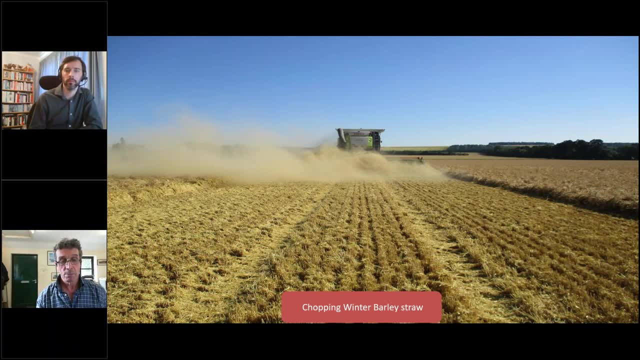 because the low cn ratio they break down much more quickly and don't tie up nitrogen. um, just going back to cereal and just whizzing through a few slides showing the problems over the years: chopping winter barley straw there a few years ago, um, you can see down the left hand side. i don't know if 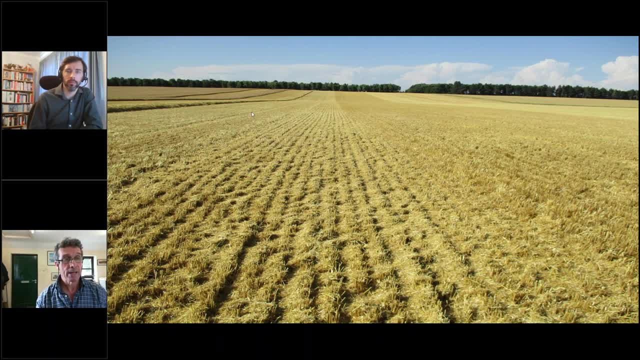 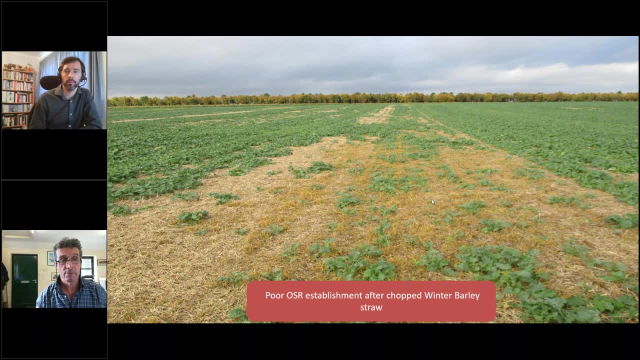 you can see my pointer. we left a straw swath and bailed it and subsequently direct drilled or seed rape. that's the or seed rape establishment over the whole field. that's actually after we redrilled it. the first establishment was really poor and then we drilled it for a second time. 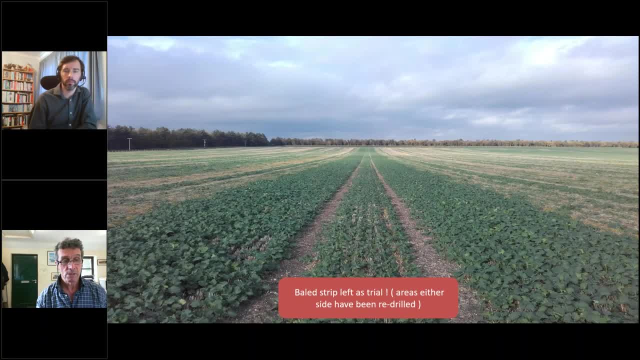 that's the area in the field that we bailed the straw swath. so you can see, we ended up with a crop on the bulk of the field which was a bit half at half mast, um, compared to the fantastic crop where we took the straw off. and you do have to ask yourself the question: you know this, this crop? 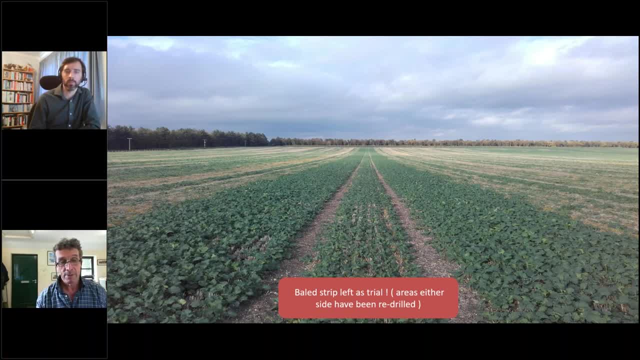 where the straw came off. you've got big high biomass crop, big root systems, good photosynthetic exudates going down into the soil. um, and you do wonder if you shot yourself in the foot a bit because you've fair enough, you've incorporated the straw on the bulk of the field, but actually 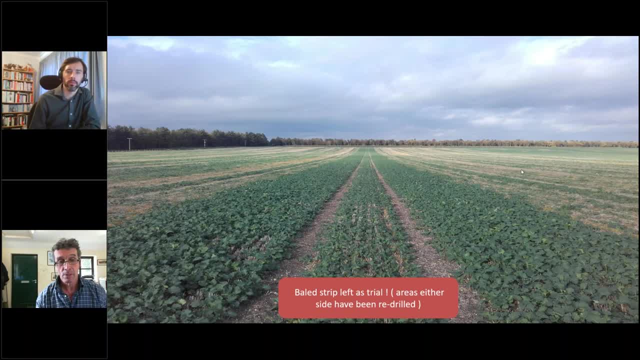 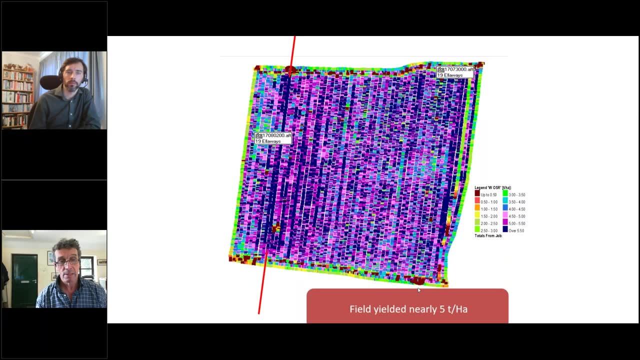 have you ended up with less organic matter in the system? um could have sold the straw and ended up with a nicely established crop of rape. the end result actually was very um satisfactory. the whole field averaged nearly five tons of the hectare, but you can see the bale strip down that left-hand side where i've got the two red lines to mark it if you look across. 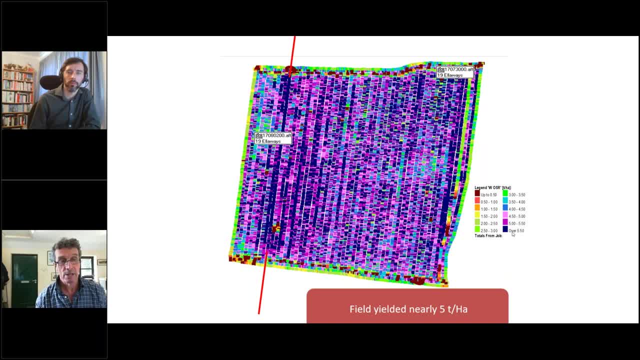 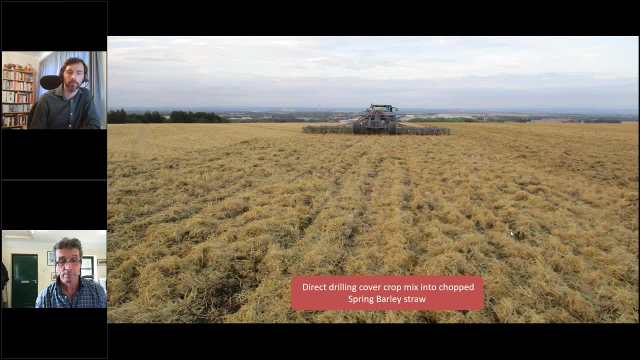 and that bit yielded well over 5.5 tons of the hectare, so it was a significant yield increase. um other issues here: direct drilling a spring cover crop, a cover crop mix into chopped spring barley straw, um basically wasting my money on the expensive seeds in the mix because only the mustard 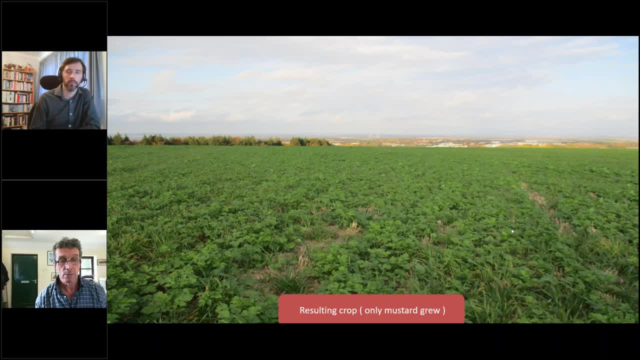 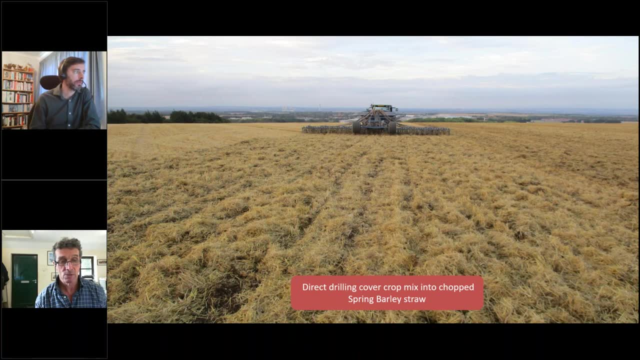 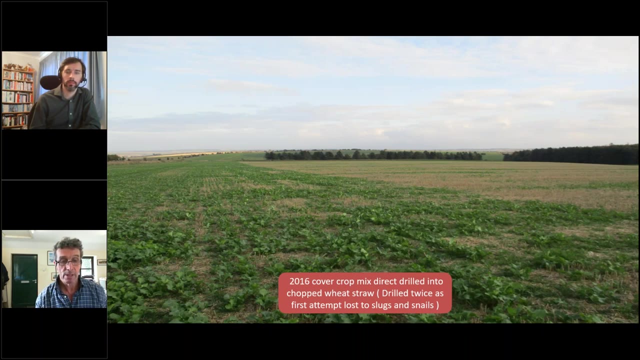 grew? um, everything else failed. it's it's too harsh an environment we we've found over the years to try and plant things into the spring barley straw. it's such a massive straw breaking down um uh, 2016, we had to drill this field twice um first attempt lost to slugs and snails. 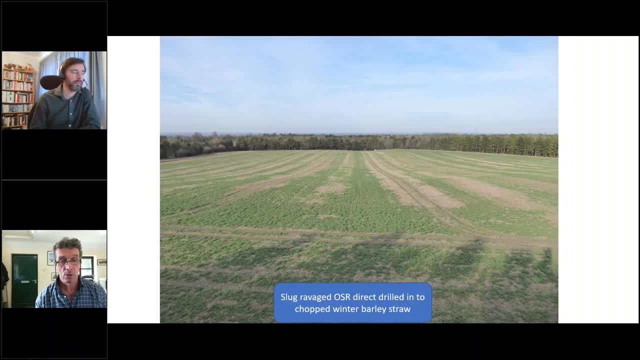 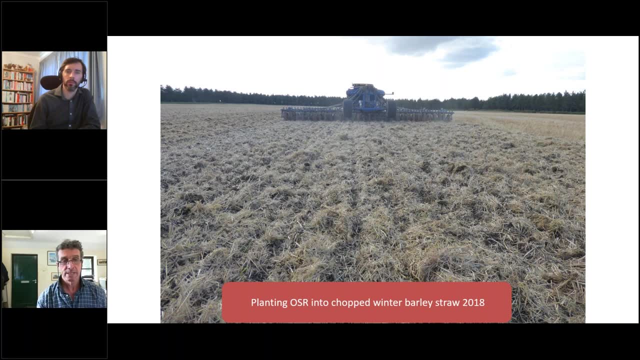 um all seed rape last year, direct drilled. after chop winter barley straw, again slugs have ravaged it um. over the years, we've learned to cope with these straw residues. though this was in 2018, drilling all seed rape that was the resulting crop in mid-november. the only issues 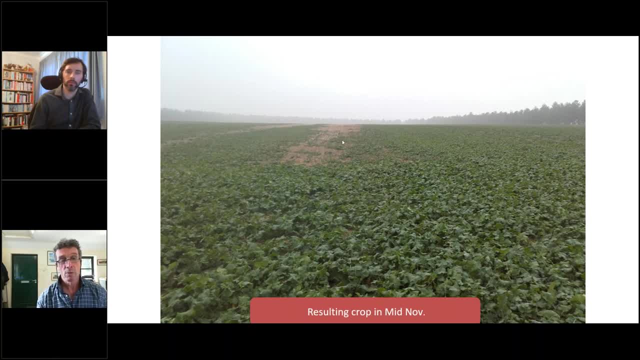 in that field, just two strips down the middle of the field where we were combining the winter barley. uh, combined too late in the evening and the chop quality deteriorated. um, where we have poor chop quality we find real issues with establishing rape. um, but generally we're we're coping with. 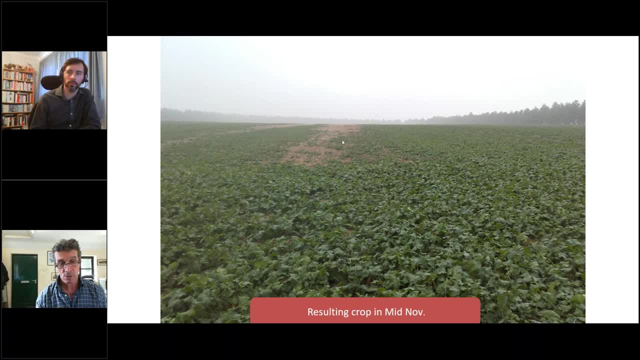 these high straw loadings. now we're doing lots of multiple rolling passes to ensure soil to seed contact and i think, as my soil system gets used to a big load of high cn ratios going back in the whole time, it's just gobbling up the residues uh, more quickly and easier than it did in the past. 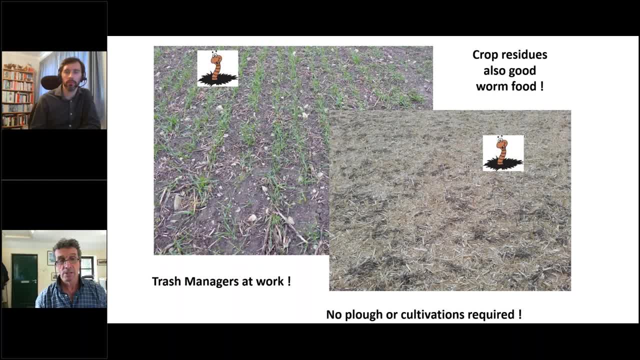 obviously the other thing with a lot of high cn ratios- uh residues on the surface- is they're really good worm food. so, um, i'm feeding my nice deep burrowing earthworms and we see all over the farm earthworm middens everywhere and they're basically doing the incorporation for me. um, 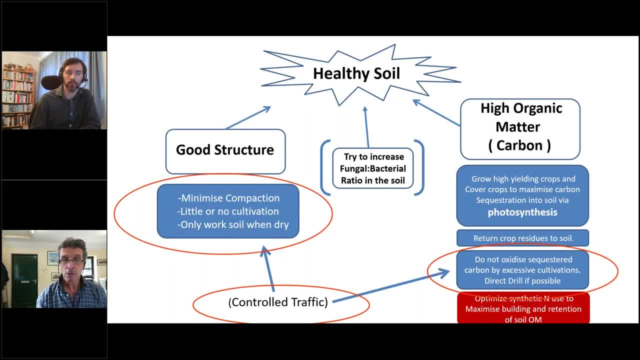 right. next one quickly, um looking at both sides of the equation here: or building organic matter and structure. on the structure side, the minimizing compaction and not cultivating um. that's where controlled traffic feeds in and also not oxidizing the carbon that we've sequestered. 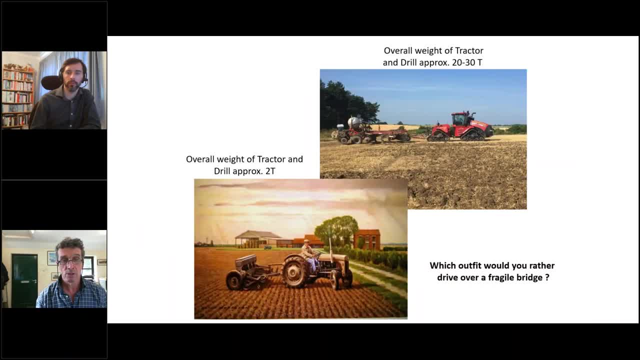 so this is how we do our control traffic system. first of all, if you just think about where farm machinery's gone, 40, 50 years ago you might have a tractor and drill two or three. turn down in the left-hand corner, little old gray fergie. um, nowadays you're talking 20 or 30 ton for an outfit. 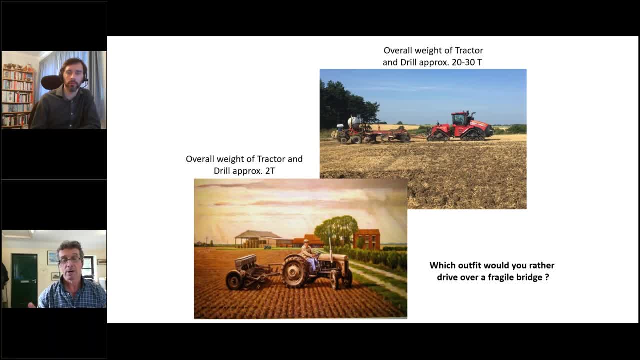 and, fair enough, they're on white tracks. the ground pressure is low on the surface, but it's the overall axle weight acting down on the ground on the soil is still a big problem. you know, imagine a flimsy, sleeper bridge over a dike in the fens. I know which one I'd rather drive over the fragile bridge. and it's just thinking about. 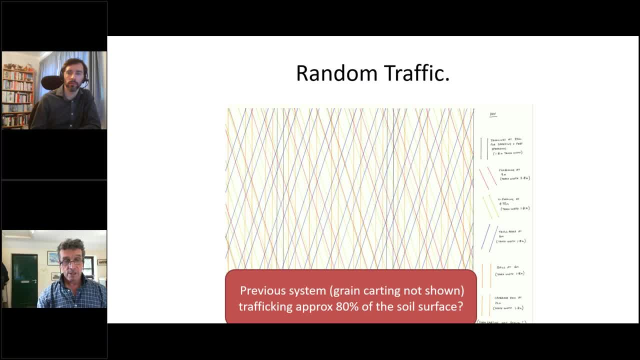 the big axle loadings on the soil. what we used to do on Hendred Estate is basically, like a lot of other people: multiple width implements, drive in different directions all over the field, so we were trafficking 80% of the soil surface. now we've got everything set 10 meters wide on multiples of. 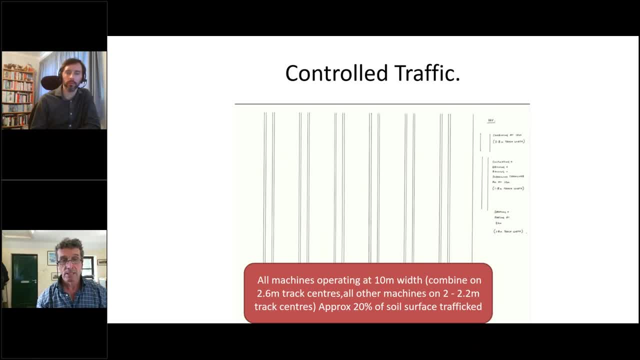 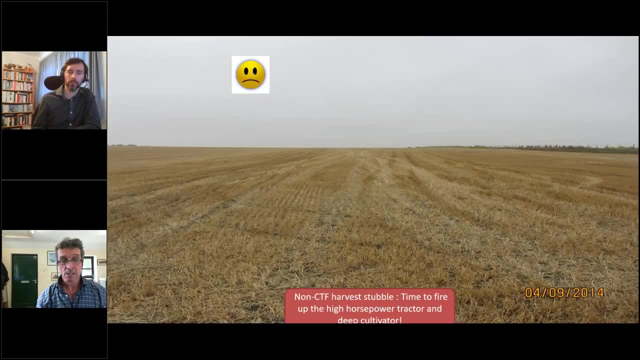 10- 30 meter tramline widths and we've turned our trafficking on its head. instead of trafficking 80%, we're trafficking 20%. this is what it looks like in the field that's a neighbor's farm after harvest, so lots of compaction damage randomly all over the field. they've got to cultivate to. 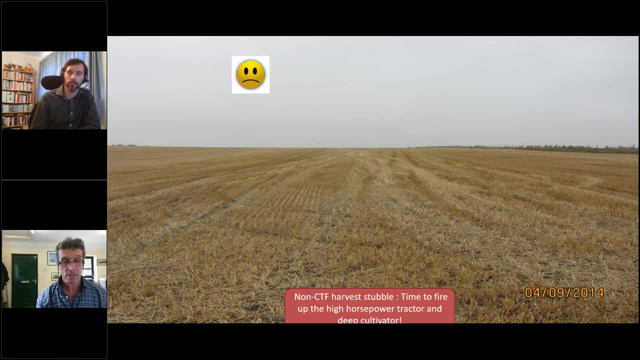 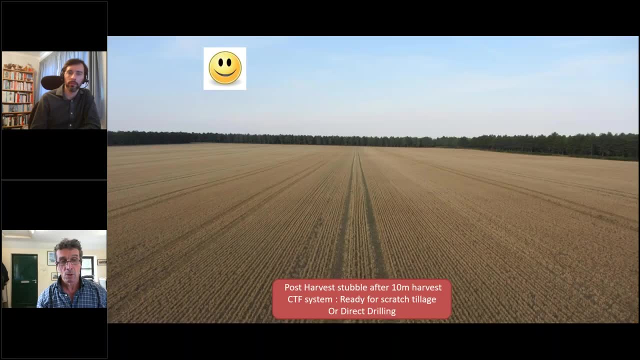 alleviate that, obviously letting carbon out the system in the process and damaging fungal networks and all the other problems with cultivation. our system next door, basically 80% of it untouched, and where we have got, if you can see my pointer there, between every 30 meter tramlines there's a couple of infills where we're trying to grow crops, if they're. 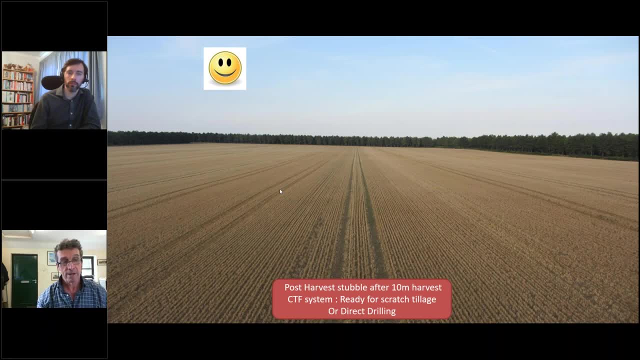 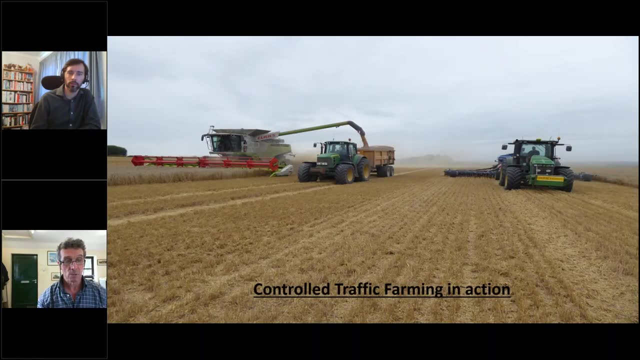 compacted, we can just run down with a two-leg subsoiler and just alleviate that compaction without touching most of the soil surface. that's what it looks like in practice. vehicles also sort of using the same set of wheelings, that's drilling a cover crop type behind the heart of the combine. 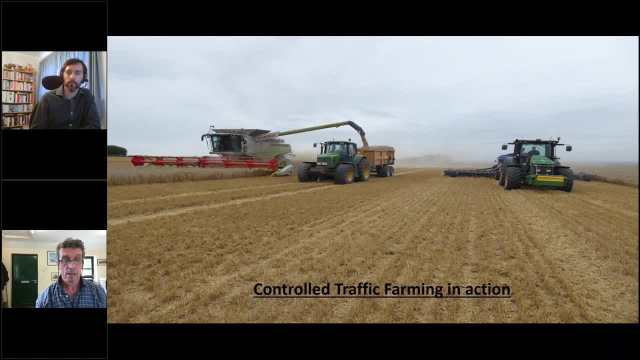 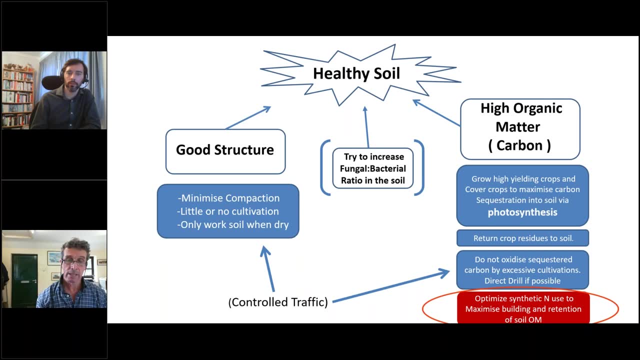 basically the drills: chasing the combine out of the field. the last big topic- nearly finished now- this is one that I'm sort of increasingly. we could talk about this for hours but I've only got a few minutes. I'm increasingly motivated by this optimization of synthetic and to maximize the building retention of soil organic matter. if we 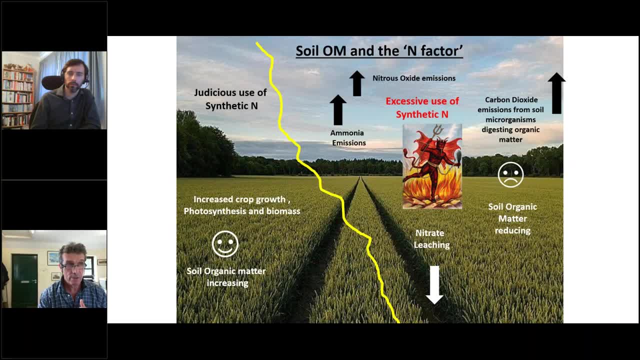 think about it. here n is. it ends the elephant in the room really that people don't really talk about that much in relation to soil organic matter, and it's a good guy. it's a bad guy if you think about it. judicious use of synthetic n one side of the balance. it's fantastic you're increasing crop. 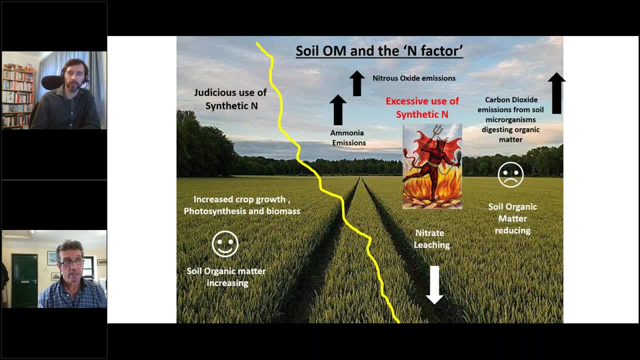 growth, photosynthesis, biomass, building soil, organic matter, and I think that's where, in a lot of ways, conventional farmers can hold their heads up high compared to organic farmers, because we are growing 12 ton crops of wheat instead of four ton crops of wheat and we are putting more. 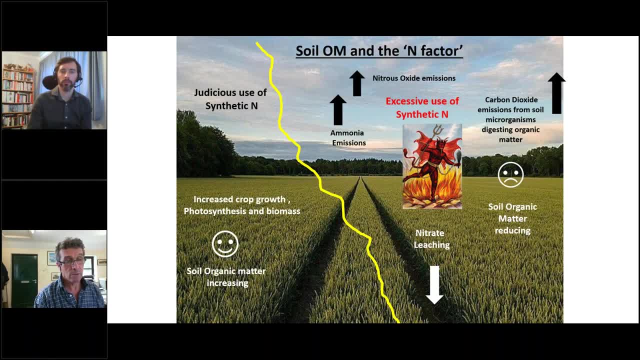 carbon into the soils with judicious use of n. so it's good. but then if you tilt the scale too far away and go into excessive use of synthetic n, you start to get lots of problems. obviously, if there's a lot of synthetic n in the system, soil system and the soil biology is looking for carbon to balance. 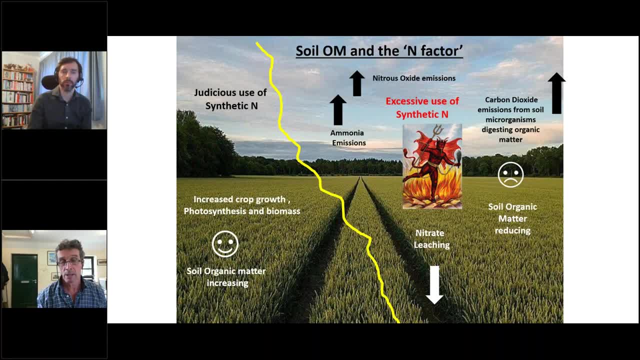 at the CN ratio. the only way you can really get it to start eating soil organic matter, and then we start to get carbon losses into the atmosphere. we get the other and the soil organic matter is ultimately reducing. we also got problems with nitrate leaching, ammonia emissions, nitrous oxide. 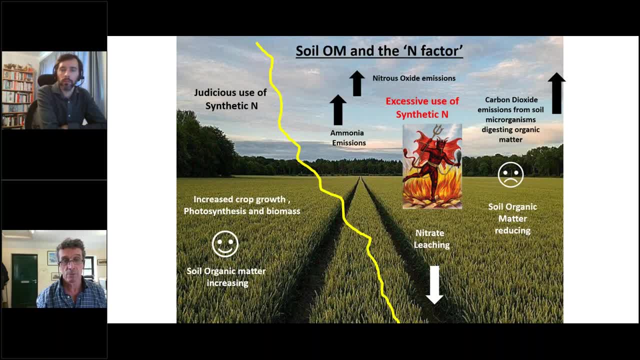 emissions, which they're all big problems with excess nitrogen, but we can't really go into those. so I think really there's a new paradigm with um, soil nitrogen, uh, with sorry synthetic nitrogen. I mean, in the old days, farmers, we're sort of always talking about optimizing synthetic end use to maximize economic, economic yields. but I think if we're really serious, 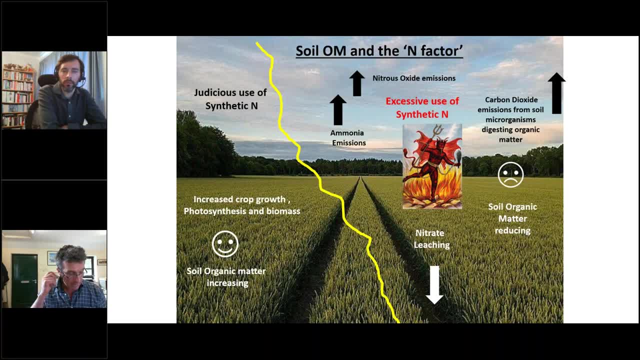 about climate change and maximizing soil organic matter. we really need to think about um optimizing synthetic and for maximizing organic matter accumulation in soils, which is a slightly different level of synthetic end, which would be much lower down the scale. um, I think there's a lot of work to be done. 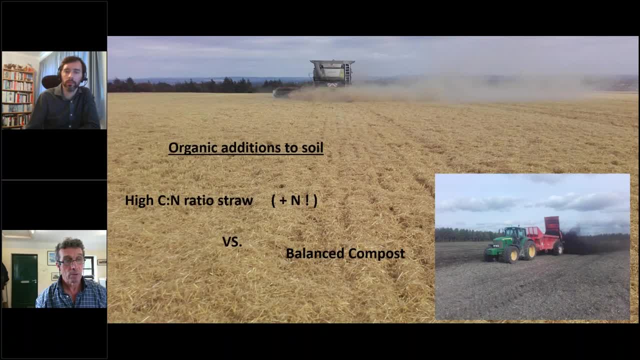 on this concept? um. just two little side points to do with n? um there's lots of things to talk about n and it's all about increasing end use efficiency, which we try and do in lots of ways on the farm. but two other little side points which I think are quite interesting: um I often think about this. 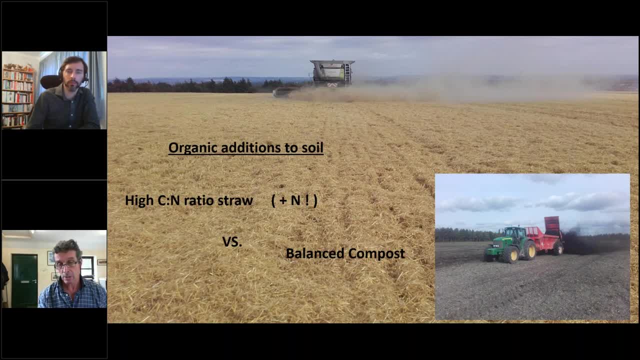 concept. if you're putting a balanced CN ratio material into soil like a compost, a nice balanced compost amendment, I often think that the soil biology just sort of thinks: oh, Mr Farmers, basically just added soil to soil. there's nothing for us to do, boys, we'll just roll over and go back to sleep. but where I'm putting a big load of high CN ratio straw, 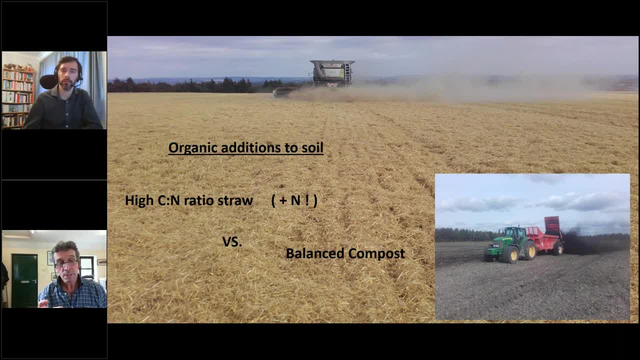 into the system and if I'm putting synthetic end with it as well, the obviously the soil biology has got to wake up to digest that um straw and obviously it'll utilize the synthetic end to equalize the CN ratio. so you're turning synthetic N into organic N in the bodies of the soil organisms. 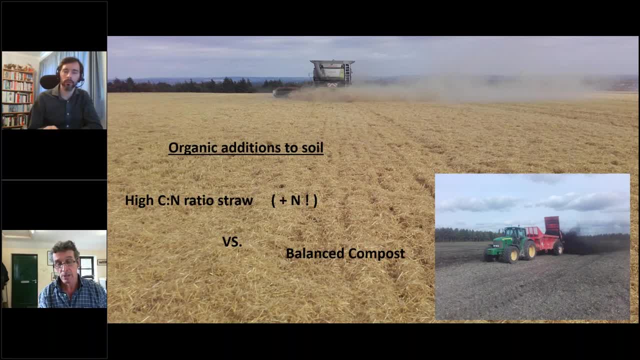 and obviously eventually these are rotting down and it's becoming organic N that becomes slowly available to crops. but in the meantime you're you're sort of locking up synthetic N, stopping it leaching over winter and turning it into a much better format, and the whole thing I always 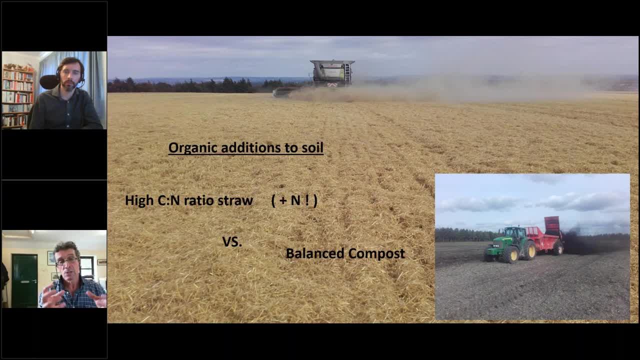 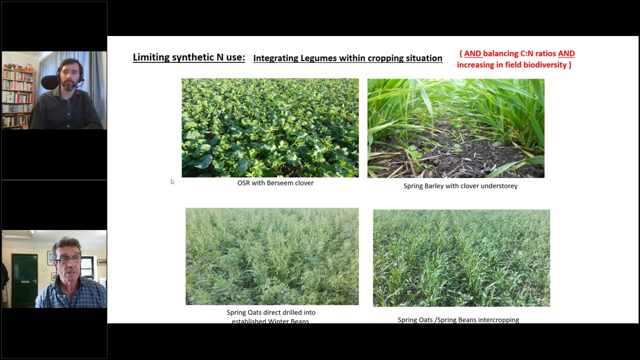 think is maybe stimulating. as long as you've got enough soil biology, they're stimulating it to all work rather than just putting something that's nicely, nicely balanced into the system. just a thought um the other thing with nearly finished, now I've got very two slides um limiting synthetic end use. we're sort of on the farm, we're trying to integrate legumes. 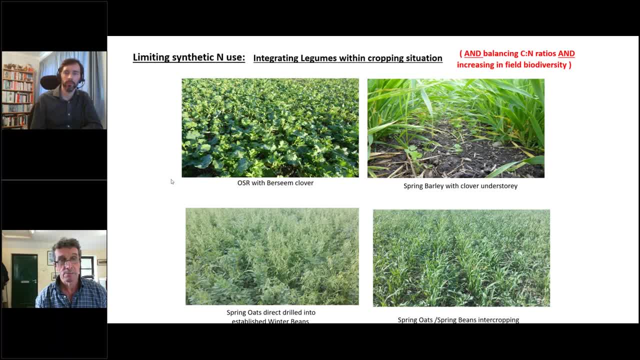 within the cropping situation and obviously this has got lots of benefits because it's also balancing CN ratios in the system um and improving sort of nitrogen lockup situations and improving the sort of overall carbon use efficiency and also increasing the infield biodiversity, as I spoke about earlier, and getting diverse riser spheres in the system um. so companion cropping- 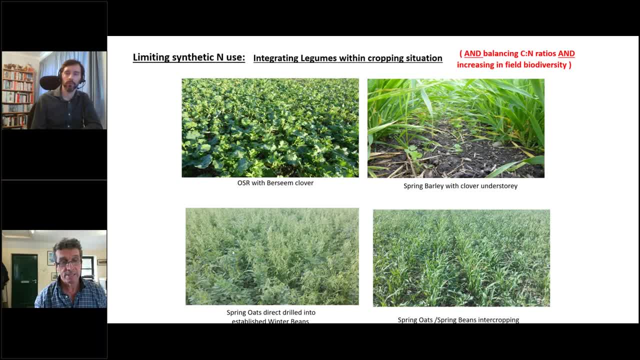 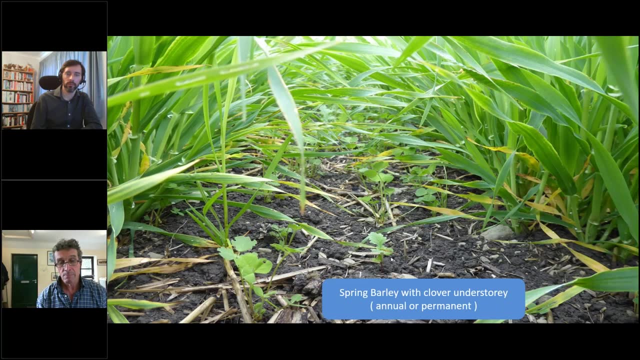 um works with all seed rape. it's very difficult. we've tried to take it to harvest with beans and oats- very difficult to harvest and very difficult to separate them. so it's work in progress. this sort of clover understory is more interesting. and again, two last quick points: um playing around with. 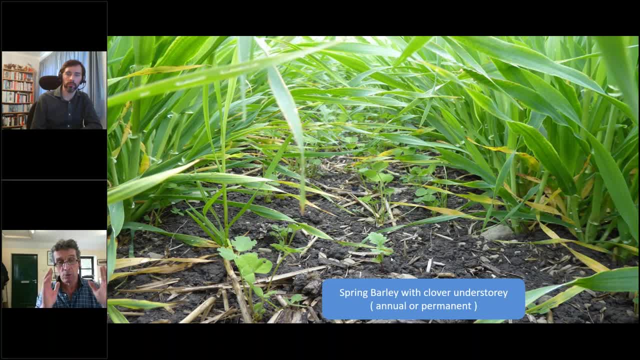 a either an annual or permanent clover understory and planting crops- annual crops- into it. the permanent one, we found, doesn't work very well. it's very, very difficult because the clover gets too established and it out competes the annual crop. but I think, for example, planting a clover understory with the spring barley and then when you harvest, the 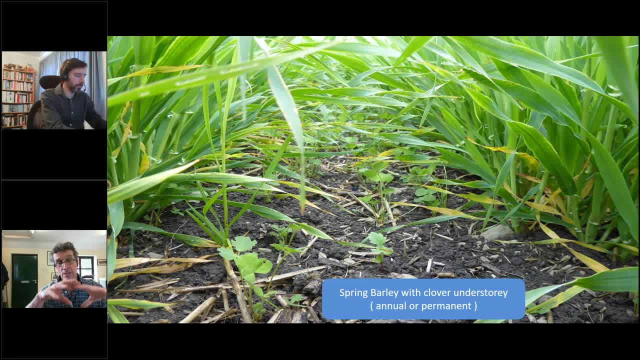 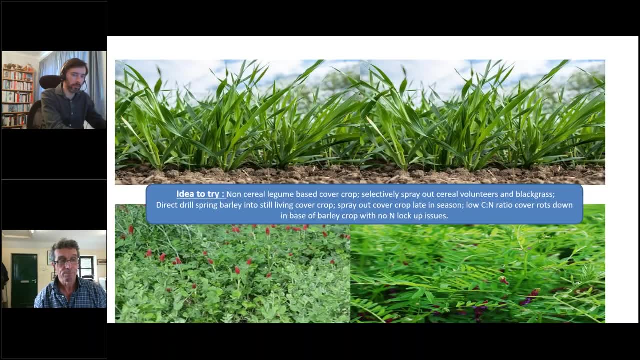 spring barley, you've already got living green material to harvest. that solar radiation in August and September is a useful concept that we're playing around with. and also the other idea is putting a non-serial legume based cover crop in in the autumn and selectively spraying out the cereal and black grass out of the system and then direct drilling the spring. 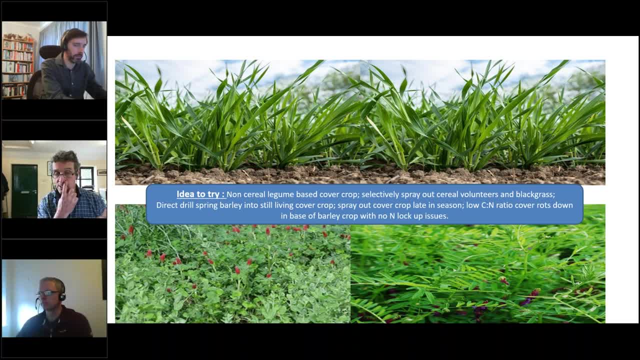 barley into the living cover crop rather than using it with sheep or springs off with Roundup and then leaving that in the spring barley crop as long as you can, probably late April, early May- and spraying it out with a selective herbicide. and that way you've got. you've had this legume cover crop in the system, growing under the spring barley. 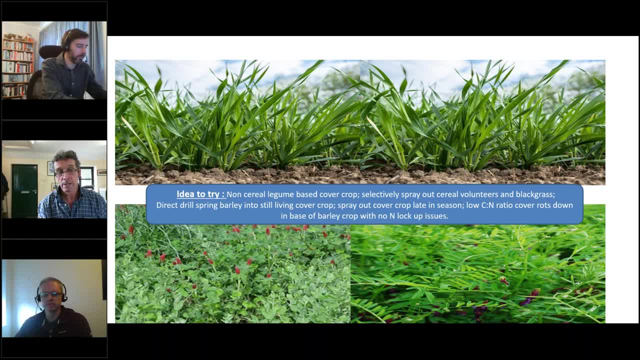 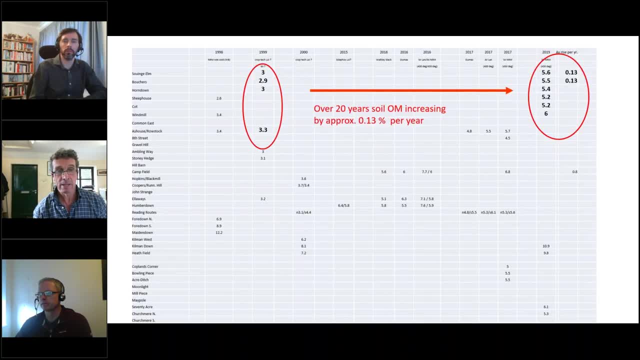 and you've got this low CN ratio cover crop rotting down and it's not locking up nitrogen for the growing barley crop and getting assimilated quickly. I think I better leave my last two slides other than just two quick comments. over the years we build with building soil organic matter- I reckon over 20 years. it's a rate of about. 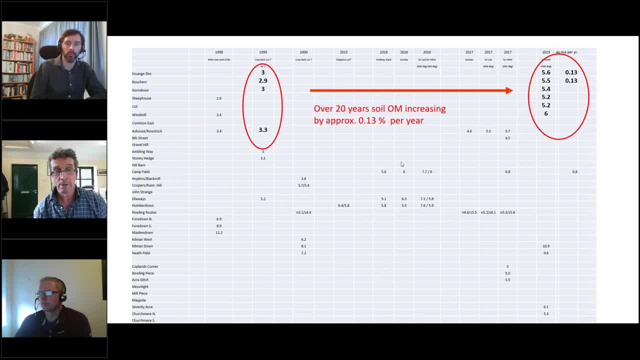 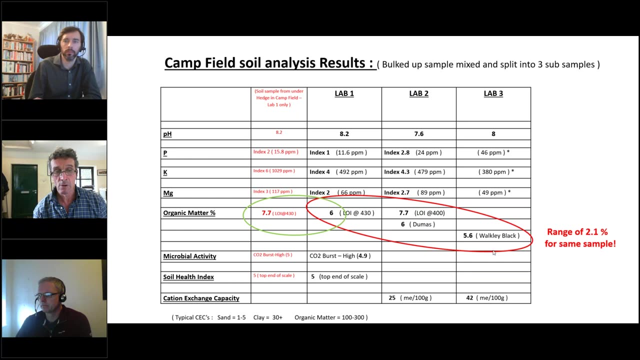 0.13 per year. so it's not a quick process and we're not matching the four per thousand initiative yet. but remember we're not got the rotational layers in the system and we've not got organic amendments. and the last slide was just a point on be careful of soil. organic matter testing- uh, one in the red. 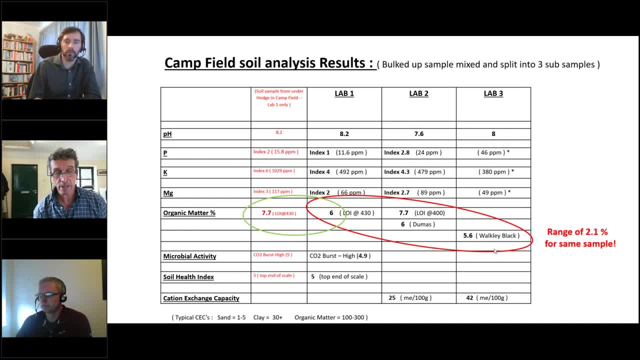 oval, one sample effectively to three labs and four different soil tests, a range of 2.1 percent. the more interesting thing is the green oval, which is um a soil sample from a field and a source sample from under the hedge next door to it, sent to the same lab on the same day with the 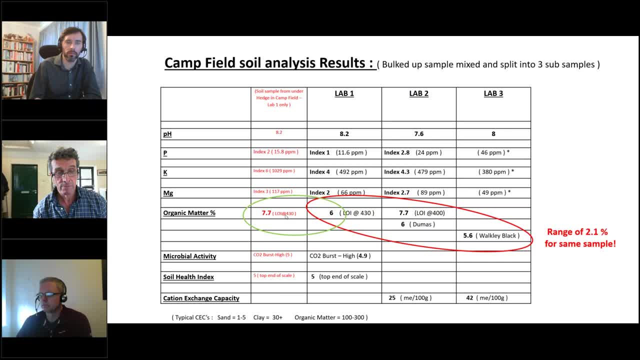 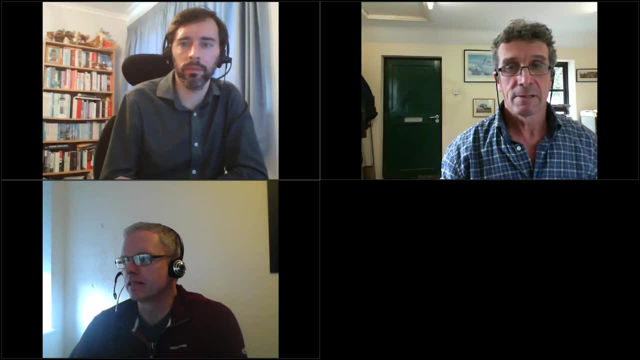 same test, so it shows me what I'm trying to achieve. in the fields I've got a sort of natural soil organic matter of 7.7 under the hedge but I'm managing to achieve six in the field where I've got a cropping system going on. thanks, brilliant. thank you, Julian. some great insights there into. 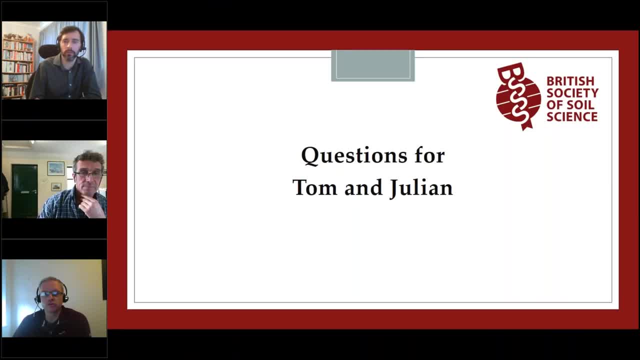 the application of the science and and some great questions that you posed as well, I think. um, so Tom's been monitoring the questions. can I hand over to yourself, Tom, to try and get through as many as we can? yeah, thank you, Bruce. yeah, so we've got a few minutes to get through some questions. I've tried. 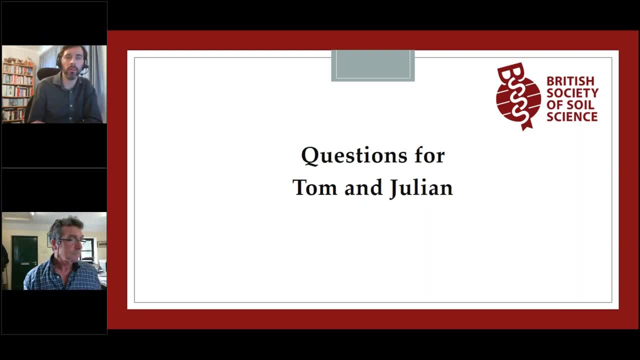 to type some answers to individual questions as well. um, I'll give Julian a break and answer one myself, and then I'll I'll hand one to Julian. um, but Israel asks: can you differentiate between the microbial necromass and the microbial biomass in the soil? are there methods to separate them? so so yeah, there's some quite long um. 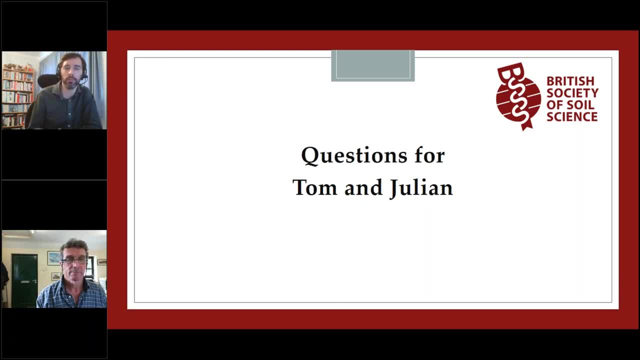 long-standing methods that we can use to um to measure microbial biomass. so typically we extract the soil with um, with a salt solution, and we can do that with by splitting the soil into two halves and one half. we would fumigate with chloroform first to kill all the microbial biomass, and that 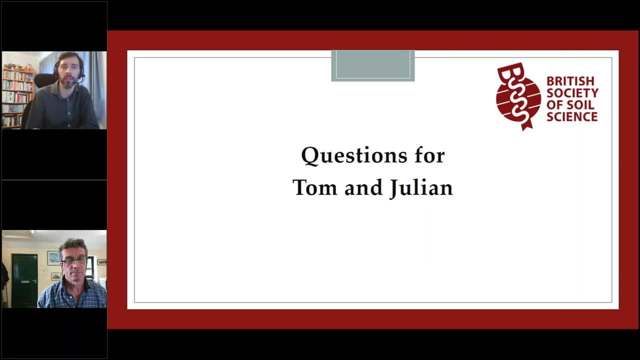 releases all their carbon and that differentiates the living versus the dead microbial community um in the soil. um I can hand one over to to Julian, I think so. there's a question here, um about whether returning crop residues into the soil causes pest issues such as slugs. so 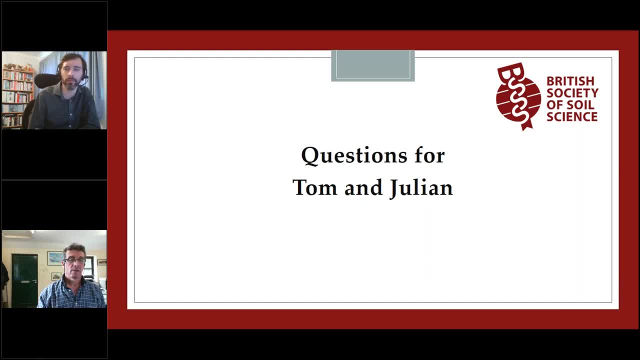 do you see these issues, Julian, and what might you do to resolve them? yeah, I mean, as you saw in some of those pictures, as slugs have been a massive issue over the years. for us massive issue: um, a bit of raking helps. physical degradation of slugs and slug eggs really helps well in the summer. so we 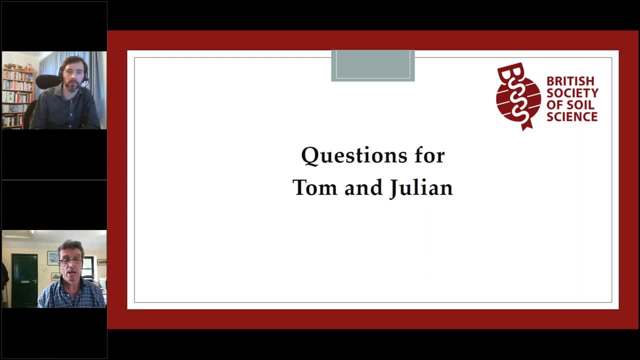 can sometimes rake if we have to. we've got a 10 meter rake that we can use. um we roll lots post establishment, which um helps consolidate. again it helps, uh, with physical slug control. we've used a relatively large amount over the years of slug pellets. I hasten to add we're using ferric. 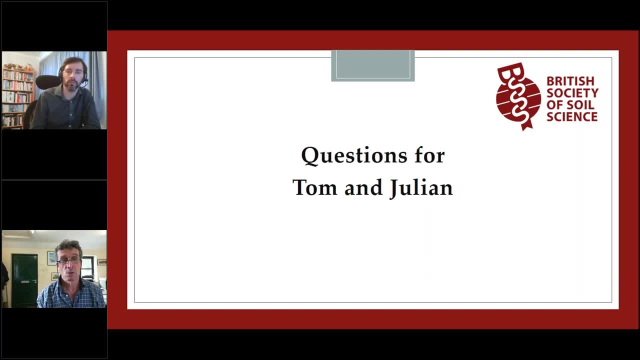 phosphate- we have been for years- rather than metaldehyde, which is kind to the soil, ecosystem, um, but also I think the predators, the natural predators, the caribbean beetles, are building up in systems. we're trying to something I haven't gone into in this talk, but we're trying to put um six. 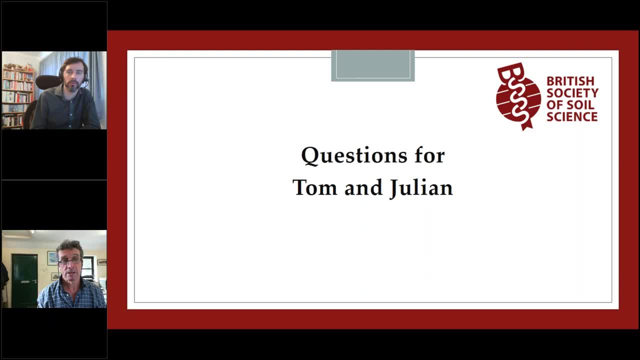 meter wildflower strips in amongst our cropping, actually down the middle of our fields as well, to give hosts to beneficials, and we're seeing benefits from that in slugs, in uh chop straw situations. so, yeah, it's getting better and better all the time, but in the early years very problematic. 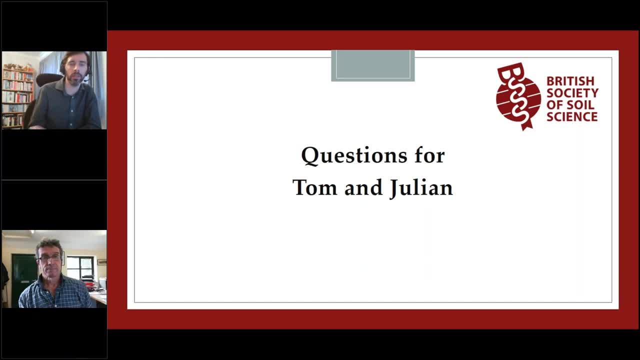 okay, uh, thanks very much, Julian. I can see there's a few other questions, um, I might uh go through as well, so, uh. so Gary asked a question, um uh saying that what I said was that all of the stable carbon in the soil is microbial necromass. but he, he points. 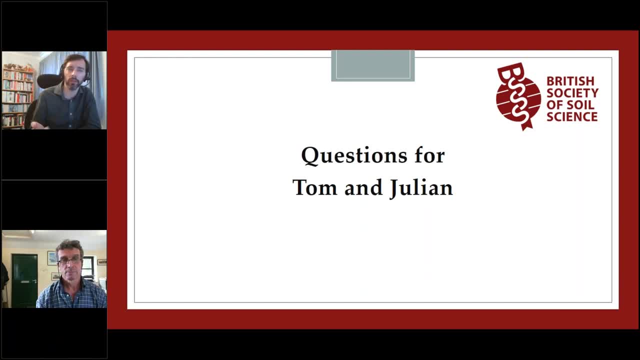 out that? is this also the case with sort of really recalcitrant carbon like um hardwood, tree wood pieces um? so I would say that yes, even in Forest systems, the the long-term organic organic carbon in soil has still broken down. is that even those Woody materials um break down? so when we look at the average age of soil organic 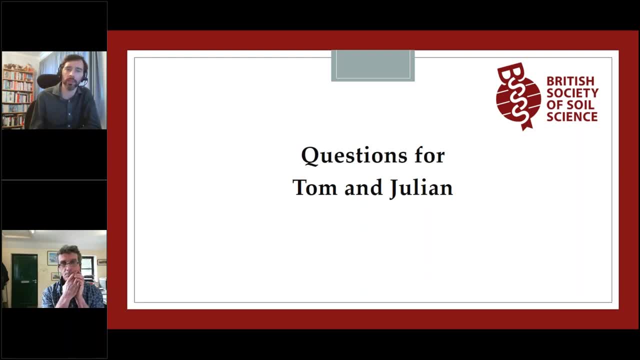 matter. sometimes it comes back as being thousands of years old. that isn't the original plant material, that's that's hung around um. however, in your comment you would also sort of mention the word water logging as well, and I guess it's a. it's just worth mentioning that um in in this talk. 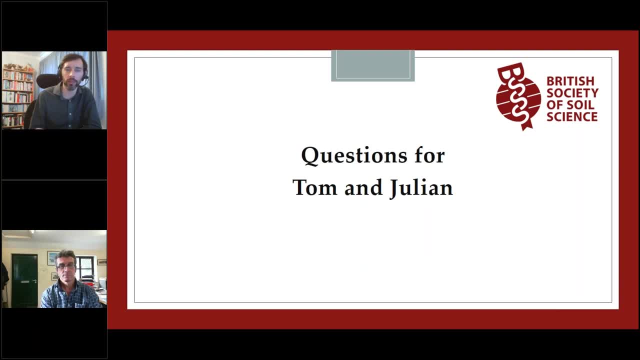 I'm mostly talking about um sort of aerobic soils. so there's a lot of generalizations you have to look at. but of course we have very different ways in which carbon is, uh is stored, for example in peatlands, where that is indeed um undecomposed um plant material. um, I do want to address a really 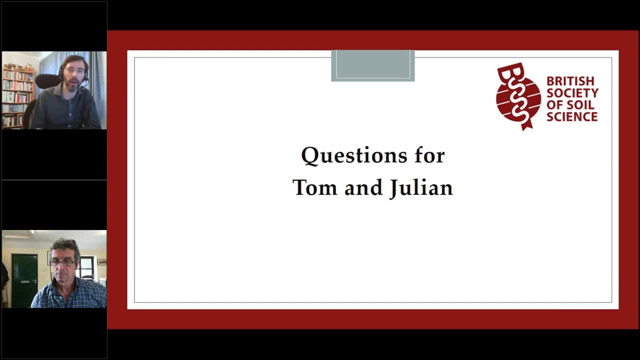 good question by Rebecca here, who's asked how, how might we encourage mineral associated organic matter instead of our aggregate or our particulate bound stuff? this is a fantastic question. it's a bit of a grand challenge, I think as well. and there's um, there's, there's, there's a lot of. 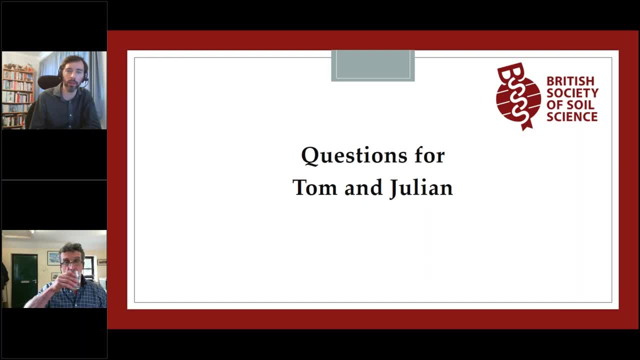 I think there's very few sort of solutions um to how we might do this, but there's some sort of off the wall ideas kind of thing so we might be able to to make amendments to our soils, um of the minerals that we know that organic matter absorbs, to. we might even be able to um to bind those minerals. 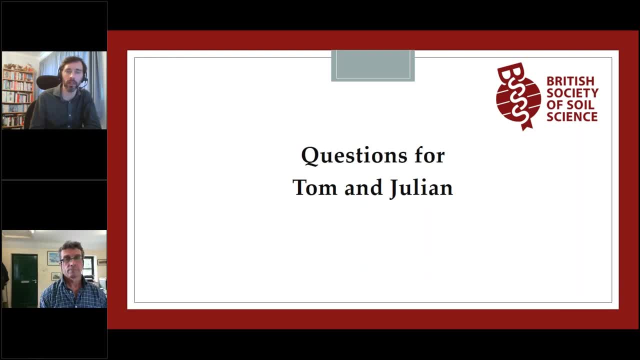 onto um surfaces that are very porous, so things like iron oxides and things like that. so there's, I think there's a a lot of um take and try kind of thing, but I don't think there's any off-the-shelf sort of methods for. 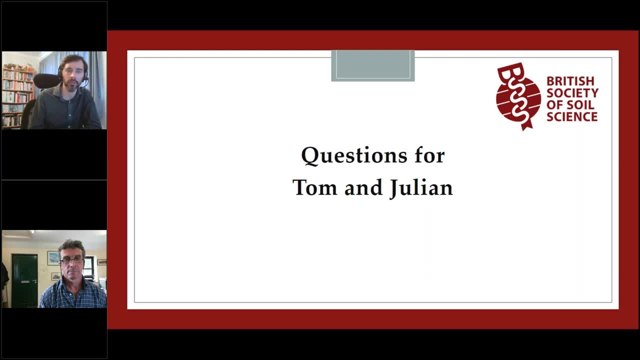 doing that, um, uh, just yet, um one for Julian, I think, and then we might make this the last one, or the penultimate one um spraying with herbicide. so is there a, is there a solution um to, I think, growing cover crops while avoiding spraying herbicides? incredibly difficult and particularly. 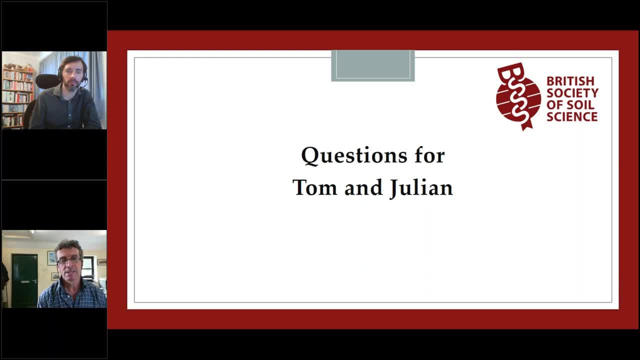 if you've got black grass in the situation? um incredibly difficult. um, I think, ultimately, if roundup glyphosate disappears from the system, we will need to think about rotational plowing coming back into farming systems um to maybe get rid of cover crop biomass. um, it's, and I don't think, a lot of people, a lot of. 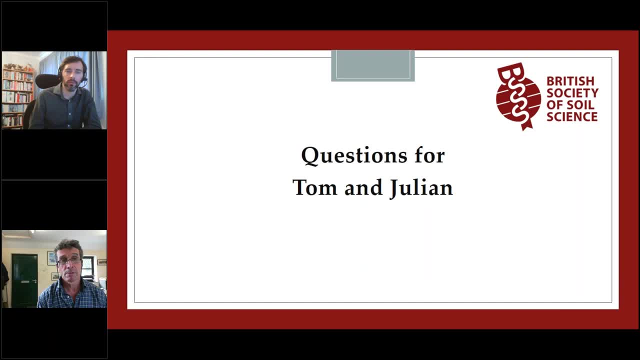 no-tillers and region AG farmers sort of view the plow as a devil's tool and I think if we've got a rotation that's majoring on building soil, organic matter and every doing everything else it possibly can, I don't think plowing very occasionally is really the end of the world. I mean, there's plenty of. 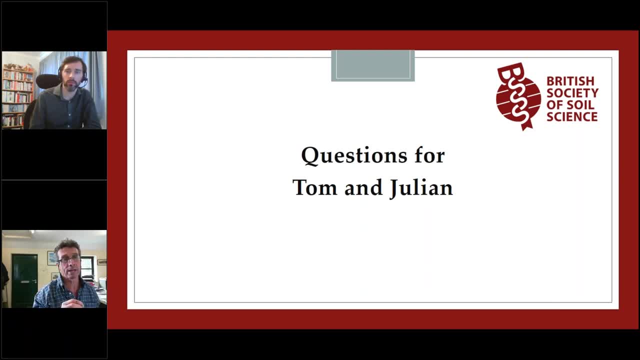 experiments. actually all plants are actually doing is just re depositing organic matter, lower down the profile, and actually it's not as bad as people think at oxidizing organic matter. but I think it's just: farming is a compromise and the herb is we're tending to use herbicide. 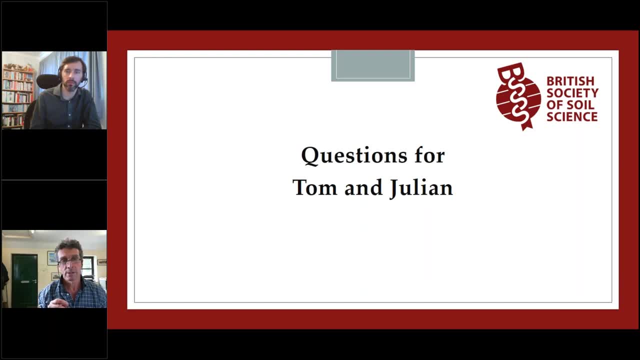 herbicides at the moment. but if we can't use herbicides, we've got to think of other ways of doing things. thank you, Julian. um, I'm just going to answer one final question, where someone highlights biochar as well. it's something I haven't talked about. but yeah, biochar is pyrolyzed organic carbon. 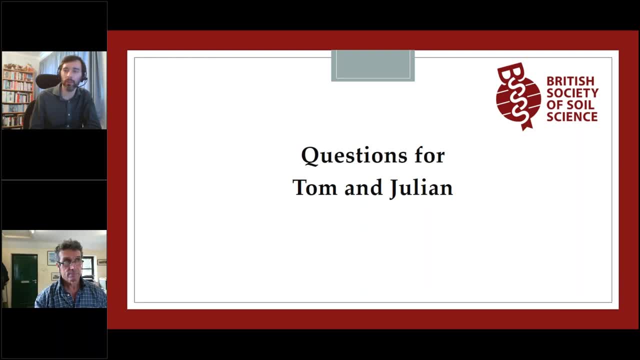 so it is recalcitrant to decomposition. honestly, I think if we're trying to um solve the climate change problem and store carbon in soils for long term, then I think the only real viable way that we're going to be able to do that in the kind of quantities that makes a really big 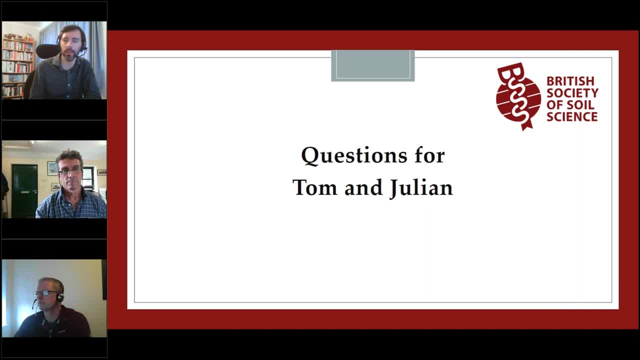 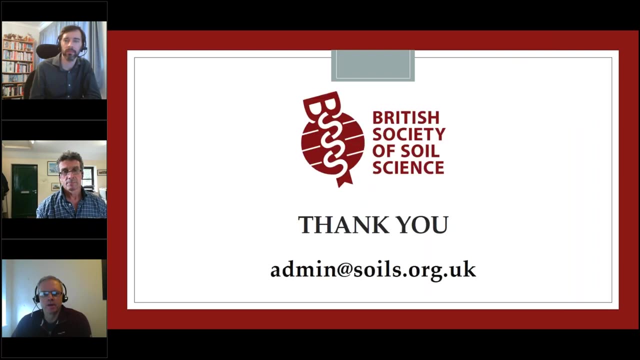 um, uh, dent in the problem is is using something like biochar, but at this point I think we're rapidly approaching one o'clock, so I think I need to hand over to Bruce to say goodbye to you and thanks for all for participating. thank you very much, Tom. um, so yeah, just finally, on behalf of the. 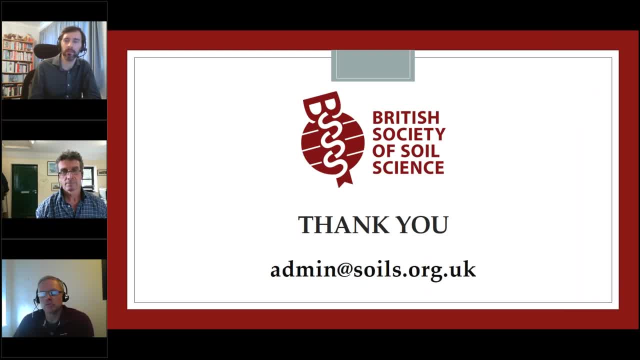 British Society of soil science. I would like to express our thanks to Tom and Julian for coming along to present today, and to Leila Froud for for coordinating sea soil support. I think it's been rather great session with some some great insights and, as ever more questions posed. so thank you all. 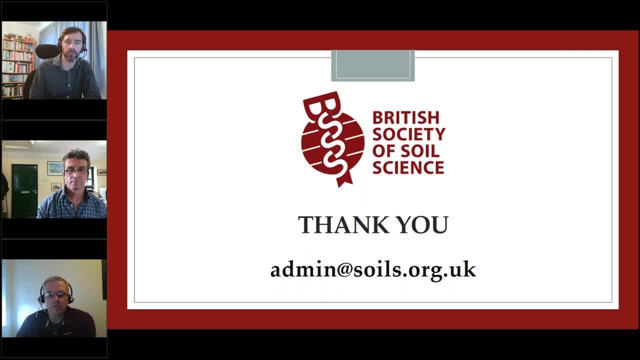 for attending. when you leave, you'll find a quick survey, a quick feedback survey, which I hope you'll take time to complete, and the recording of this video will be available after this event on our YouTube channel for you to watch again. so yes, finally, please keep an eye out on our website.